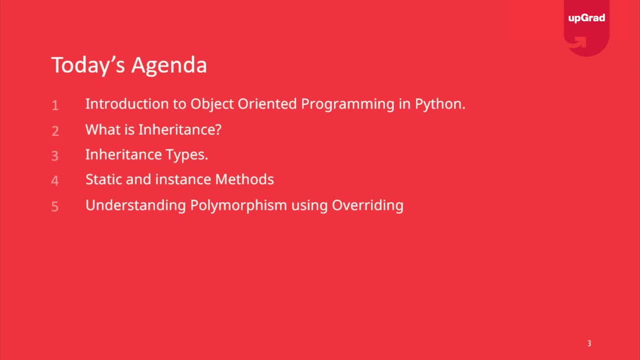 what is object-oriented programming in Python and how does it create a big difference in the programming style? Apart from that, we will be learning the various characteristics of object-oriented programming, such as classes and objects. Then we will be discussing about inheritance in Python. what is inheritance and what are its benefits? 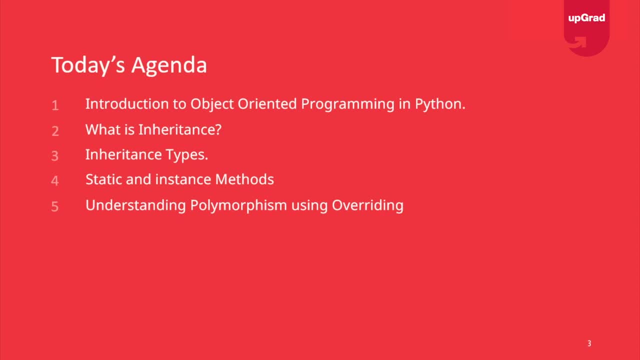 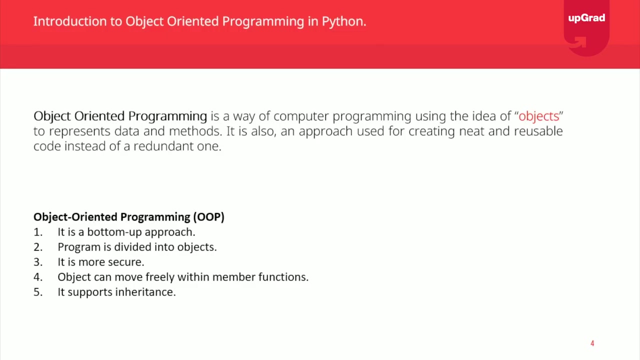 Then we will be talking about the types of inheritance, Then we will be talking about the static and instance methods And finally we will try to understand polymorphism and polymorphism using an example on overriding. Let us start first of all with understanding what object-oriented programming is. Python is a multi-paradigm programming language. 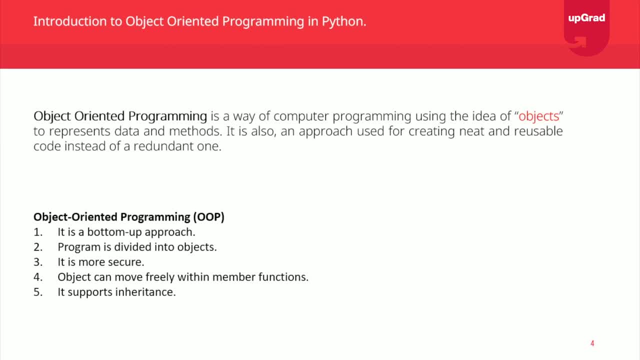 It supports different programming approaches. One of the most popular approaches to solve a programming problem is by creating objects. This is known as object-oriented programming. The concept of object-oriented programming in Python focuses on creating reusable code. This concept is also known as don't repeat yourself. 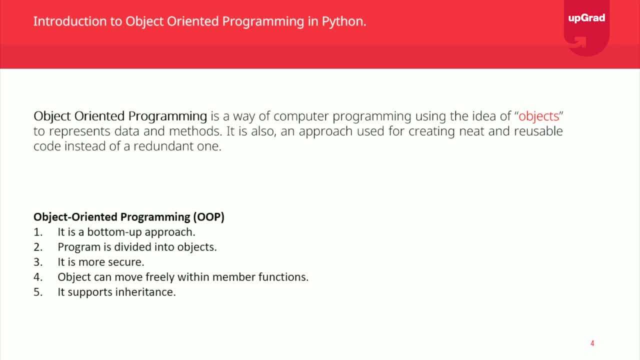 Let us put it another way: Object-oriented programming is an approach for modeling concrete real-world things like cars, as well as the relation between things like companies and employees. Op models real-world entities as software objects which have some data associated with them and can perform certain functions. Let us try to understand object-oriented programming. 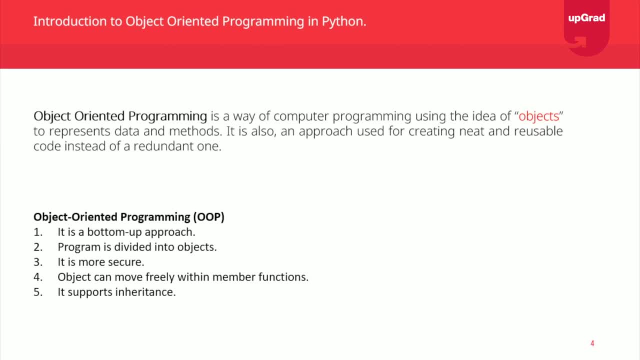 or real-world modeling, using some examples here. In order to understand object-oriented programming, we must first of all understand that object-oriented programming is used to model the relationships between objects. Objects are used to model real-world entities. so, in order to understand modeling real-world entities, 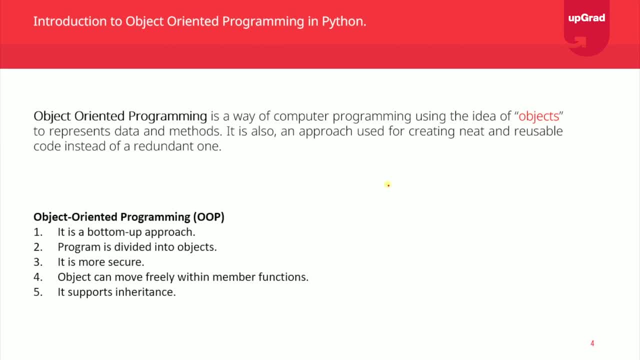 in object-oriented programming. let us take an example of real-world entities here. so let us take an example of a student here. now this entity called student must have some attributes associated with it or some data associated with it, and that can be, let's say, name, age, course. so these are. 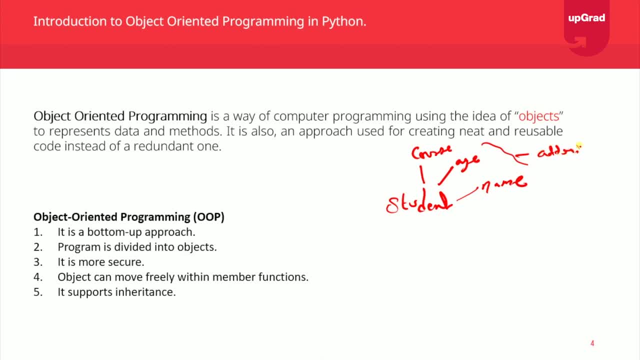 called properties or attributes. now, every student must have, or every entity must have, some behaviors associated with it. let's say, study, all right you. or let's say, take exam. so these are some behaviors associated with the entities. now, here there must be some physical representation of this entity. 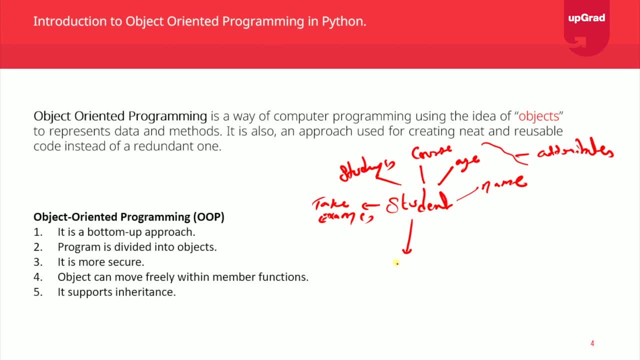 so I'll just call it, let's say, Rahul. so here you can see that here. first of all, let us understand the real-world entities here. so the real-world entities are actually divided into two parts here one is the category. here one is the category which is used to understand the behavior. 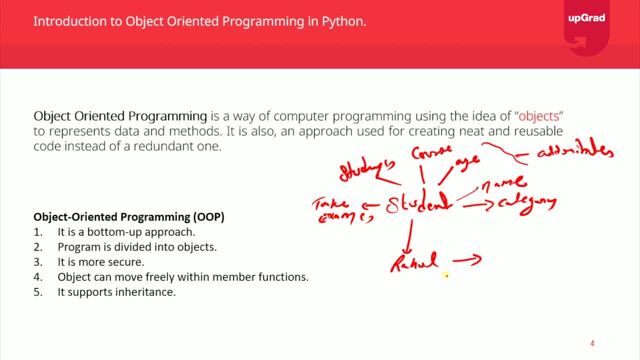 of a particular physical representation. so here Rahul is a physical entity, and student is a category to which Rahul belongs. now, anything which is physical or is tangible, and technically we call them objects. so how do we identify the objects? here? objects are the real-world physical entities, so anything which can 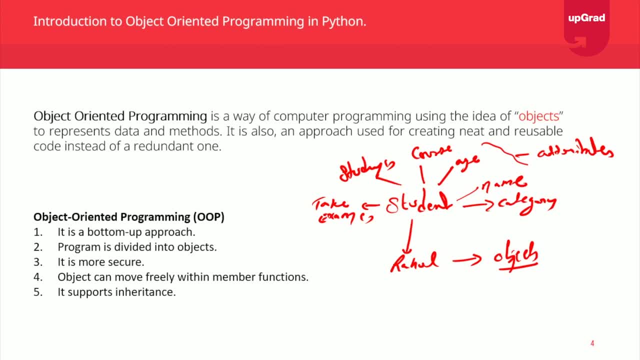 be which can come into your senses, right, so that is, objects. such an example of Rahul. now, any physical entity that exists in the real world must belong to a category. so here, in this example, Rahul belongs to a category called student. remember, categories are always logical. so here category technically can be: 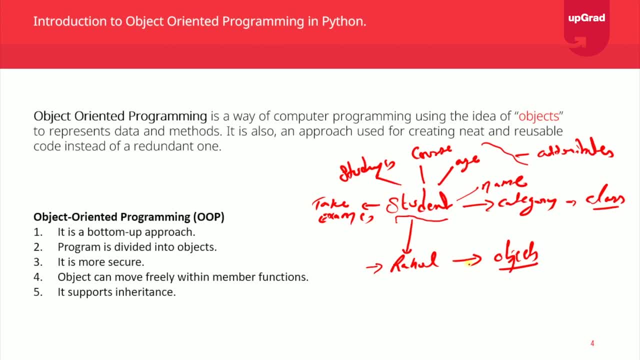 classified as class. let me give you one more example of classes and objects, or the logical categories and their physical representations. let us take an example of, let's say, car, and I'll call it. let's say of car, and I'll call it. let's say, of. 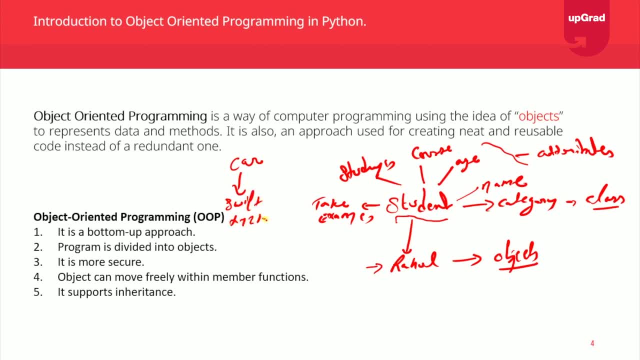 of, let's say, car, and I'll call it, let's say, of Swift XYZ 101.. So here in this example, car is a category and Swift is its physical representation. Now, in this example we must understand that the physical representation, technically, is called object and the logical 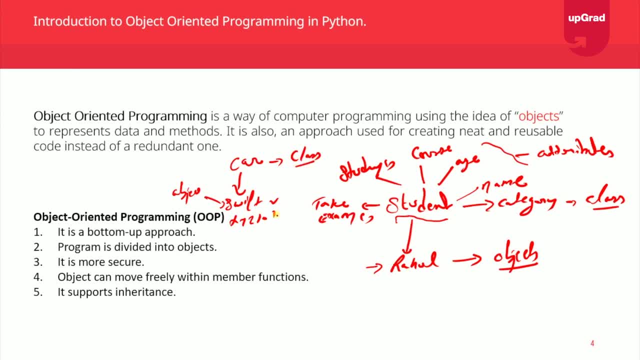 category technically is called as class. Now, this must be very much clear to the learners, that how do we differentiate between classes and objects? Now, classes and objects are the technical terms that we use in programming for representing the real-world entities. So, as a conclusion, or as a summary, the real world. 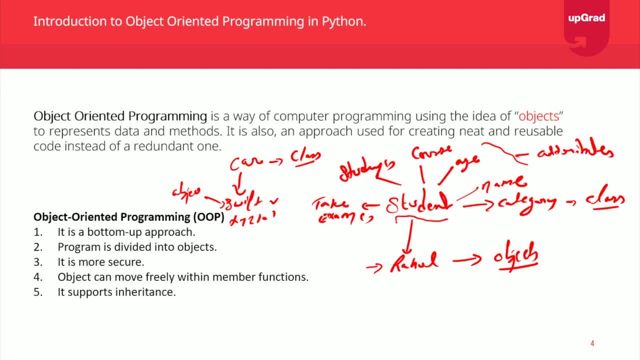 entities are divided into two parts for like for the general understanding. One is the categories, which are the logical parts, along with some properties and behaviors, And the second is the physical representation, or the you. any object which is physically representing them, such as Rahul is physically representing student and let's say Swift is physically 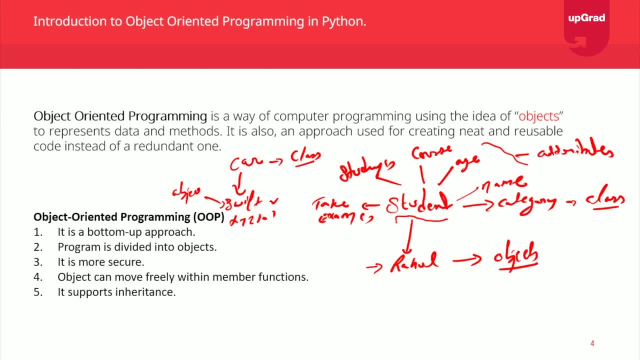 representing a car. so let us add the technical vocabulary here, and that is objects and the classes. objects in the classes are the physical, are the characteristics of object oriented programming. these are the keywords or the vocabularies which help us in modeling these categories and physical representations in programming. now, as you can see here, like object. 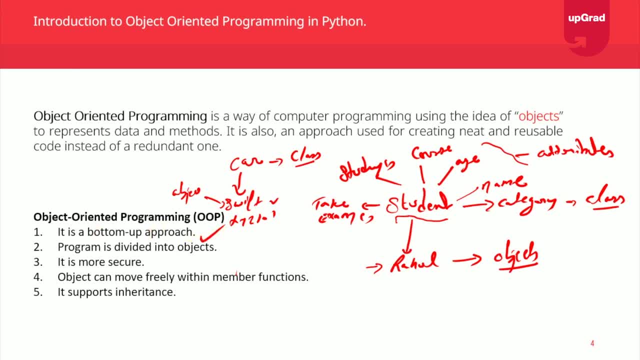 under programming is a bottom-up approach. now, what does it means? it means that first of all, we define a class. first of all we define a class, we define some functions and attributes, and then we create objects and we use them. all right, so when the code executes, it doesn't. 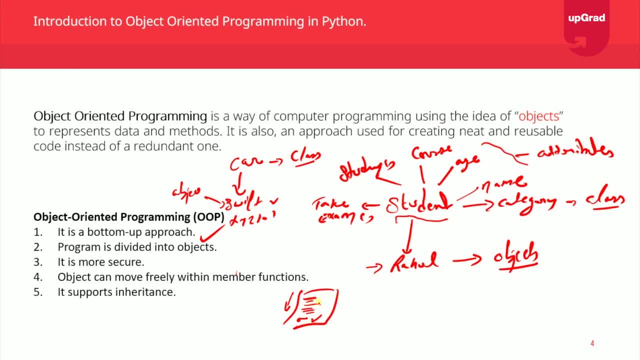 executes from the top to bottom, so the definition is given first for the particular entity. the definition includes the attributes of the entity or the behavior of the entity, and later, at the bottom, we create objects and use those members or properties. so that is why it is called bottoms and bottom-up. 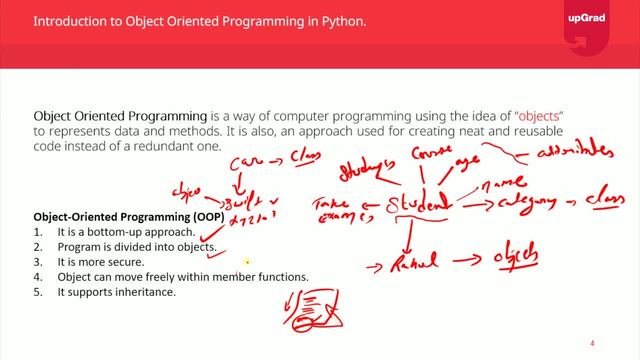 approach, the program is divided into objects, that is true. so we divide the program into various objects, such as objects of student, objects of, let's say, school, objects of, let's say, teachers, objects of, let's say, the non-teaching staff, let's say. so we divide the program into various sub models, using objects. so 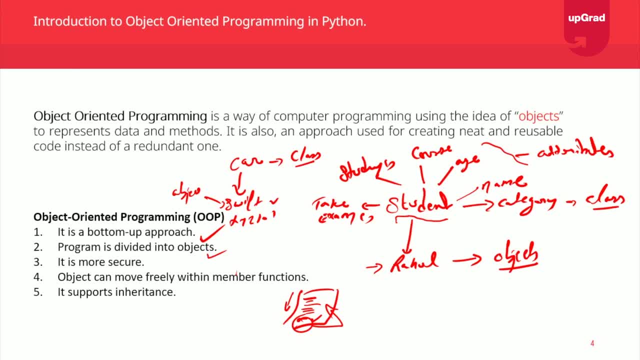 this approach of object-oriented programming brings us more security in our code compared to the other programming paradigm, which is also called procedural. procedural is the alternate or the procedural is the alternate or the process, which is the possible process. previous programming paradigm that we used to use before OOP. 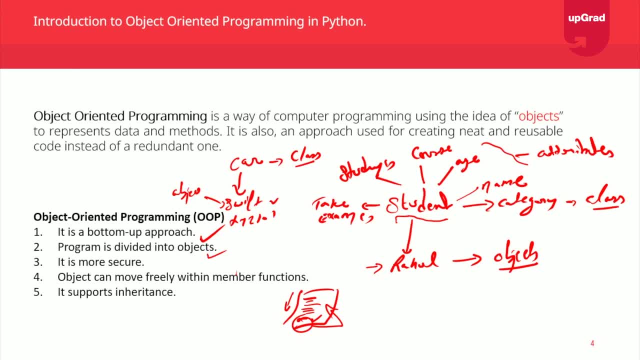 So the concepts like encapsulation in object-oriented programming brings more security in our code. Objects can move freely within member functions, so this basically means that we can migrate one object from one module to another module easily. So inheritance is one of the characteristics of object-oriented programming that is supported. 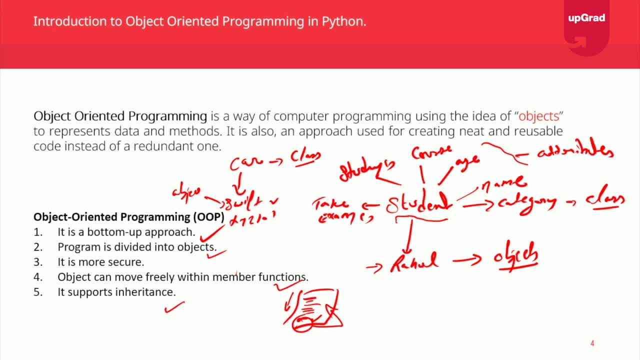 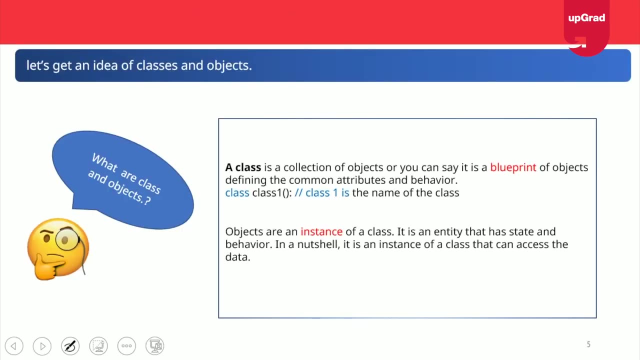 here in Python as well. So in the upcoming slides we'll be understanding what inheritance is. Now let us proceed further and let us try to understand objects in detail. So let us clear exactly what objects are. So, as I told you earlier, objects are the physical objects. 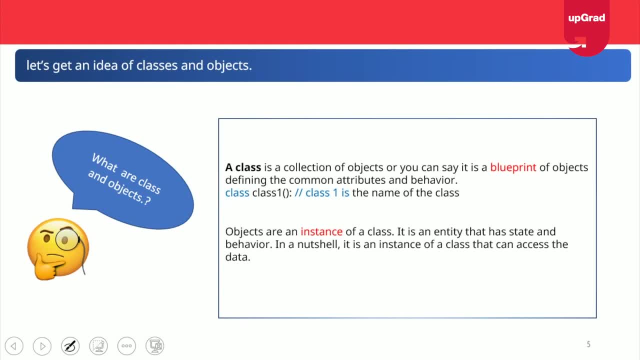 They are the physical instances, or you can say the physical representations, of any entity in the real world. Objects are basically used to access the properties and the behavior of a function of a class. sorry, A class is nothing, but it is a new data type, or you can say it is an abstract data type. 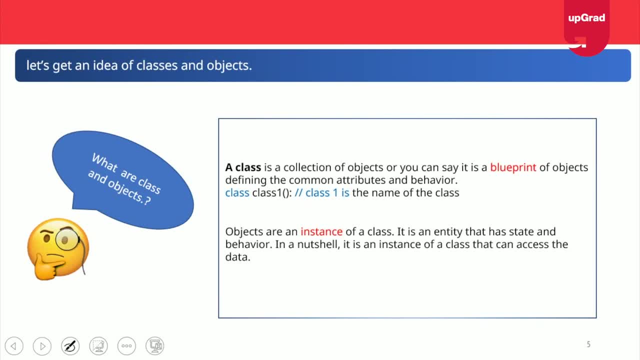 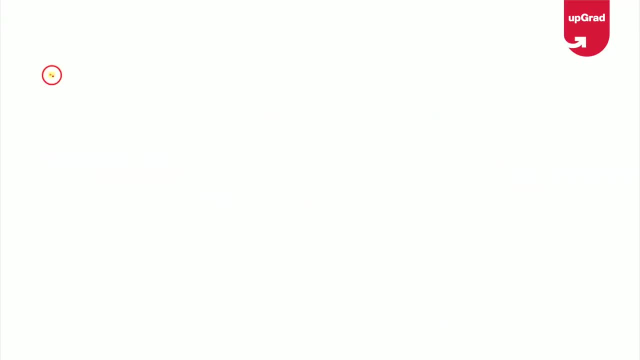 which is used to define the behavior and the properties of a given entity. Let me give an example here, one more time here, of classes and objects. For understanding classes and objects, let us take an example of a tommy and dog example here. Let's talk this way: 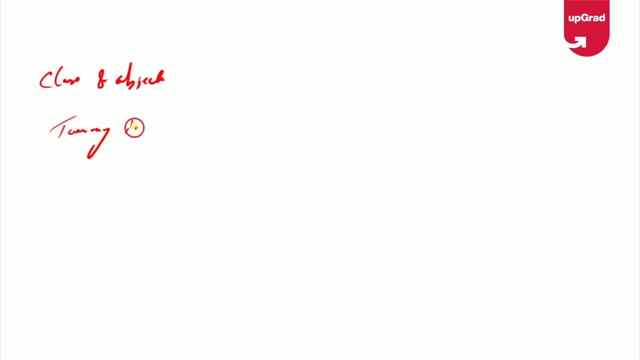 So let's say tommy is a dog and tommy barks, all right. So let's say: this is an example, this is a real world entity here, a real world situation here. So let's try to model this example into programming form or programming mode, all right. 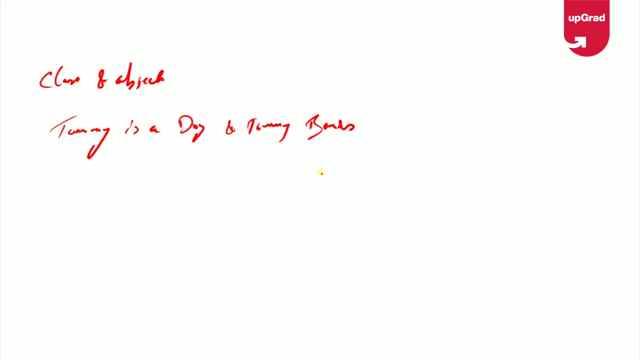 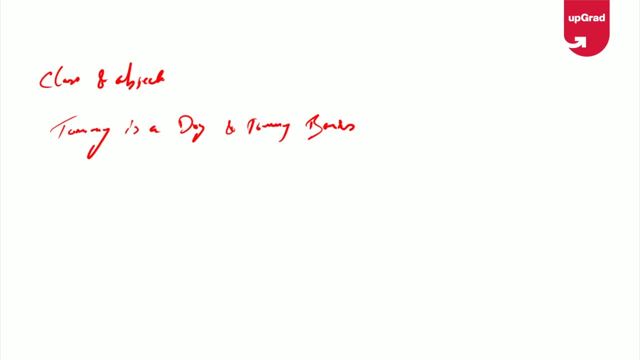 This is just a well-dejudiced, given scenario. So in this example, where I'm seeing, tommy is a dog and tommy barks. so here, first of all, we must understand: the class is an object set, So here dog is an entity. and because dog is logical, so here this is a class. 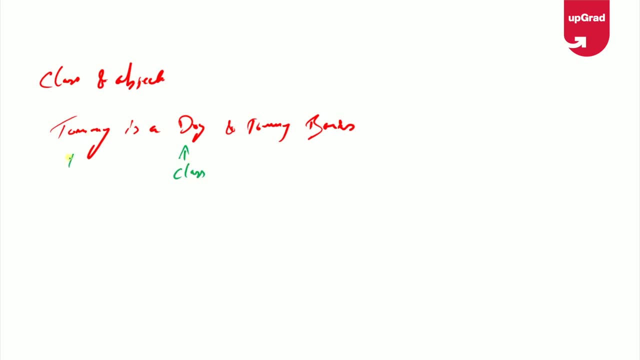 Now, tommy is an entity which is representing physically a dog here. so anything which represents a category and which is physical is called tommy, Because a dog is logical here. tommy is a class here. objects- just give me a moment. object now. okay, so here this is the name, property of this object. 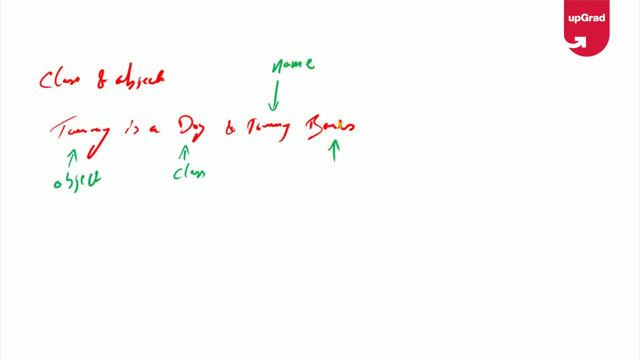 which is, let's say, tommy, and it say it says it barks. so barks is a behavior. right, it's a behavior, so i'll call it function, all right. so here you can see that. uh, here you. in object-oriented programming, first of all we need to identify the various sections or the characteristics. 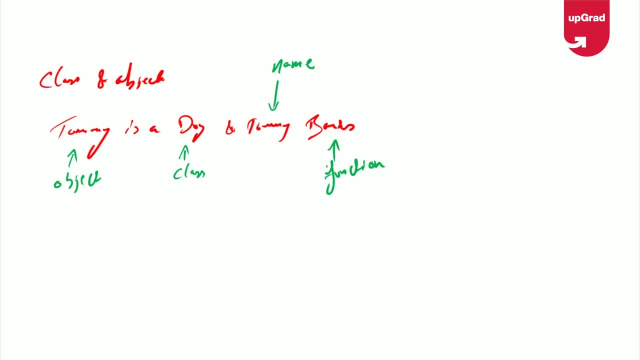 or the scenarios. all right. in terms of what is that right? so, is it, is that a class, or? or is that an object or a property? that's a name or a function or a behavior? all right, so once we have identified that, so how can we model? 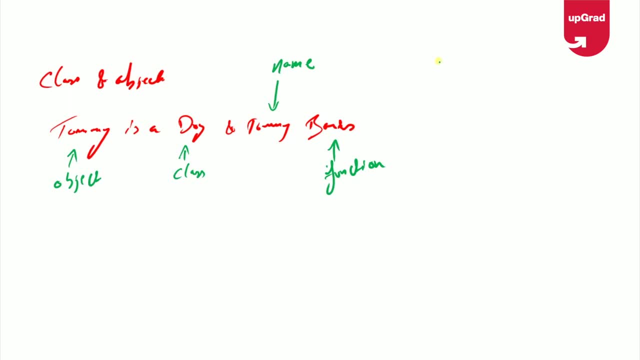 this behavior in programming. so let us look at this example in python. so so in python, oop helps you real model, the real world entities. so let us take an example here. so the class is dog, so you can see here. all right, you can see here, so i'm able to create a class in. 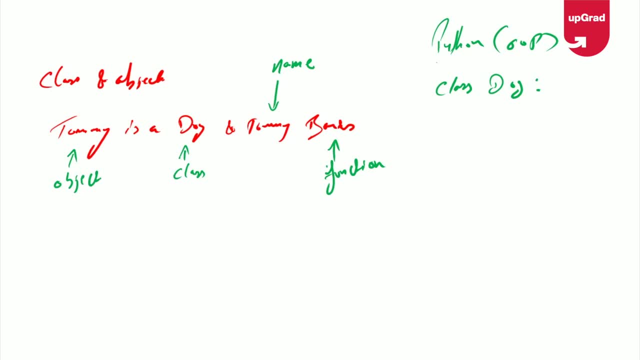 python using a keyword called class. so class is an abstract data type and we create classes to define the properties and behaviors. so when i say properties and behaviors, or properties and functions, so this means i'm talking about these two things. all right, so i can call it. let's say: name equals to tommy. 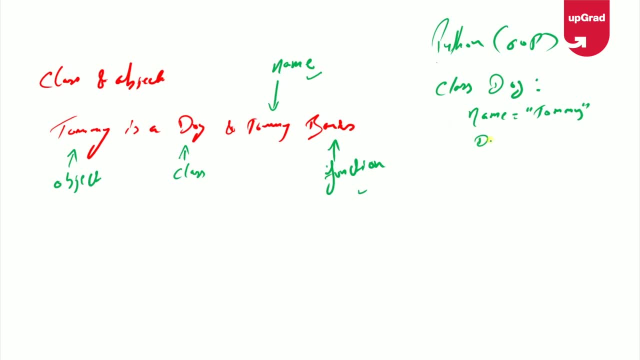 and so here i'm getting a function called, let's say, bark, and a print it says, let's say both. all right, okay. so here you can see that i've created a class called class, so i'm able to create a class. So here in this example, you can see that I'm using a class here to basically represent the properties and functions or to contain the properties and functions. right, So you can call a class like a container which contains properties and functions. that's it, right. Or you can say that it defines the behavior of the object that we'll be creating for this particular class. 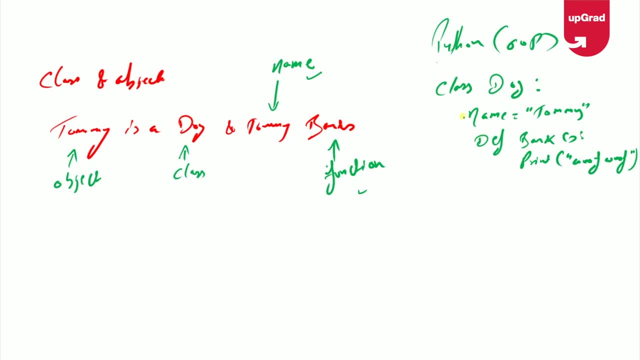 Okay, now here. now here we need to understand that, dog being the logical category, right? So dog is a logical part, So anything which is logical cannot use its properties and functions directly. That is the reason we need objects here, right? So let us create an object here. So let's say, t equals to dog. 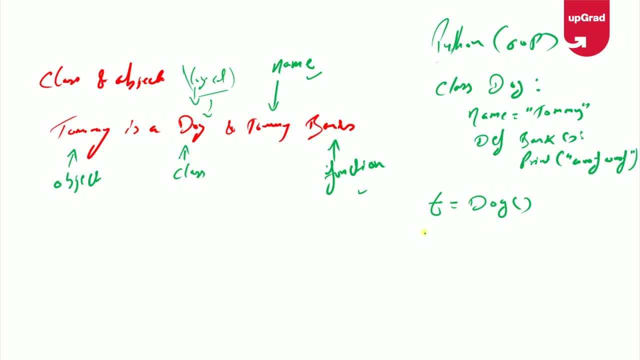 So here in this example, you can see: okay, this is the expression. This is the expression for creating objects in Python. all right, So let's call it creating object in Python. So this is an object. here, The object name is t. It can be anything, all right, And this is the expression for creating object in Python. 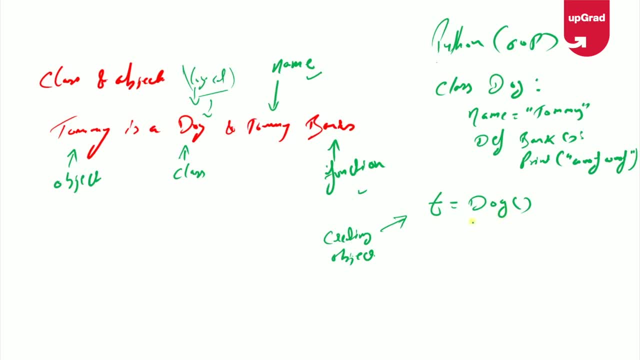 Now, why do we create objects here? We create objects to access the properties or functions which we have defined in the particular class, And that is dog here. So using t I can access name and I can call the bug function. So let us try to do that: Print tname. So if I do this I'll get Tommy as the output, all right. And if I call, let's say, tbug, So here I'm calling the function. So when you call this function, this function will be called and it will print woof, woof, all right. 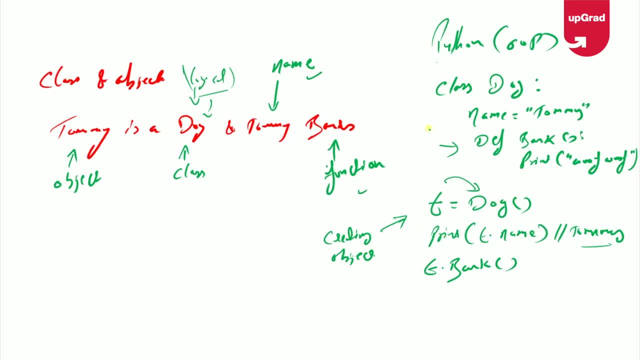 So here you can see that in this example, a class which is being used container or as a data type for defining the properties and behavior, so a class cannot access its members and functions directly. that's the reason we have, we need to create an object here. so this is the expression for creating objects in 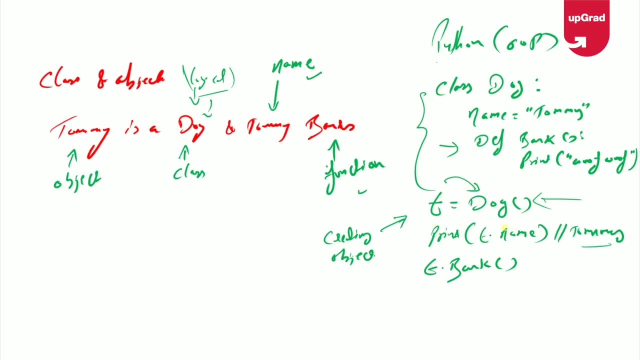 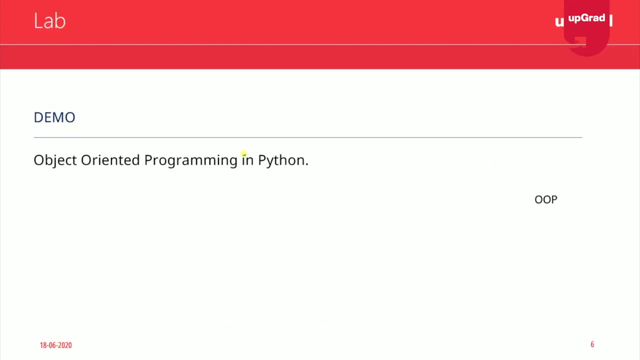 Python. once we have created object in Python, the next step is to access the properties or call the functions. alright, so here I'm. this is an example of how we access the properties, and this is example of how we access how we call the functions. let us try to understand the implementation of classes, objects, using 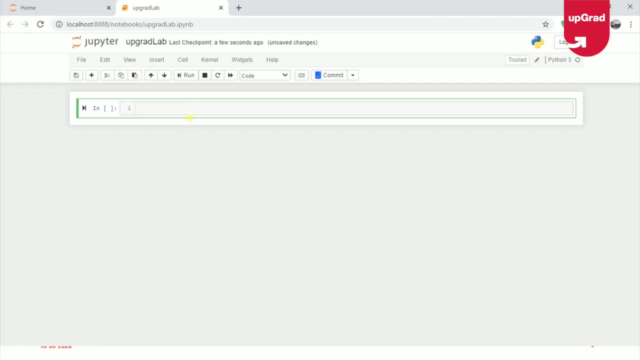 Python. so here in this example, we will try to understand how to implement classes, objects. so let us start with some demonstrations here. okay, so classes and objects are the very first characteristics of object-oriented programming. to implement object-oriented programming we must learn how to implement classes and objects and what classes and objects are. with that theory that we 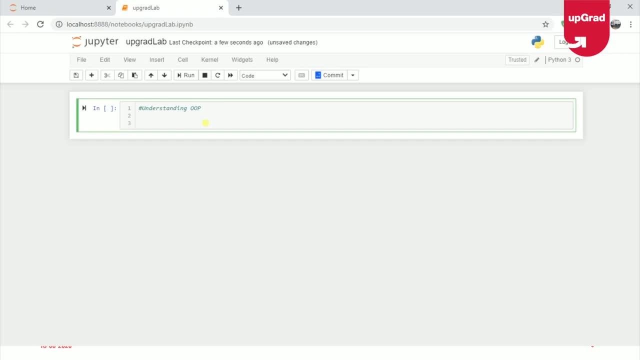 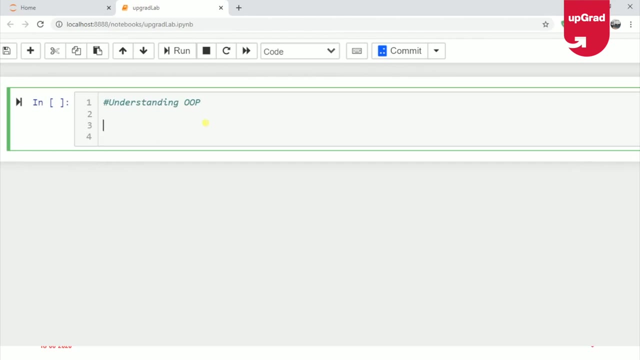 have done earlier, let us try to implement it practically here. so in the previous example I give an example of of a dog here, so I'm going to implement the same example. so observe the syntax here and the keywords that I'm using for implementing the example. all right, so here's the scenario here. all right, so let us try to implement the. 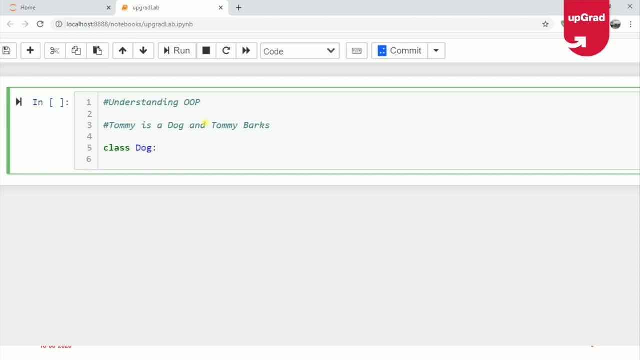 scenario. so class dog, all right. so here you can see that first of all I'm proceeding with the construction of a class here using a keyword called class. so class keyword is provided to us in Python for representing the all, for modeling the real-world entities. so here I'm modeling the 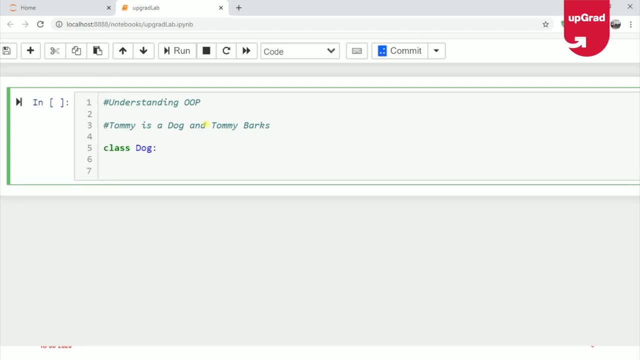 القим Disk Lite. so that is an attribute, basically. and def: bark print Woofwoof. so here you can see that I have declared a function called bark, which is the behavior actually, and what it does is it just prints a message Woofwoof, nothing else. 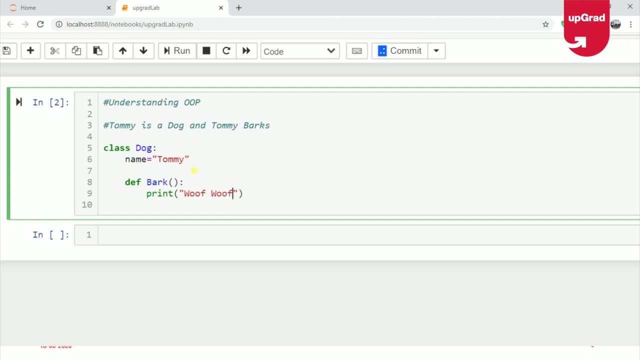 now in python. so whenever you create a function within a class, it is mandatory to create a parameter here which is called self. now, self parameter this term basically represents represents the object that we'll be creating later. now let us try to create an object here to use the properties and the functions here. so how we will. 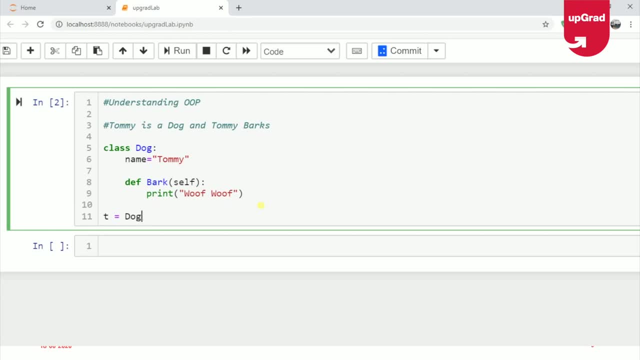 do that. so t equals to dog. so this is the expression for creating the object in python. please observe the indentation here, that this indent. this indent here basically represents that the variable and the function are within the class scope, whereas this t is not following the same indent. that basically means that this is outside the class. 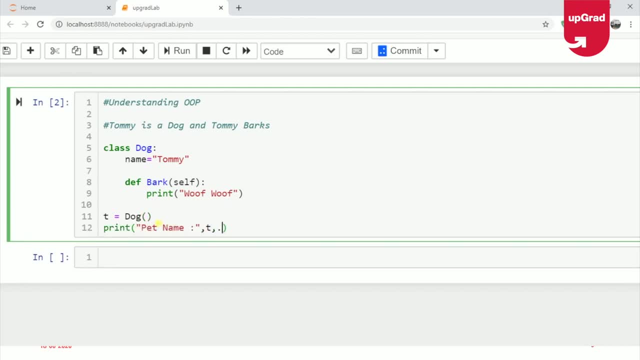 print. so if i execute this demonstration, you can see that it prints pet name tommy. similarly, we will call the function print. okay, so we don't need print for that t dot bar and we will execute this. you can see here it says uh. so we can see that it is printing the function and we can see that it is printing the function. 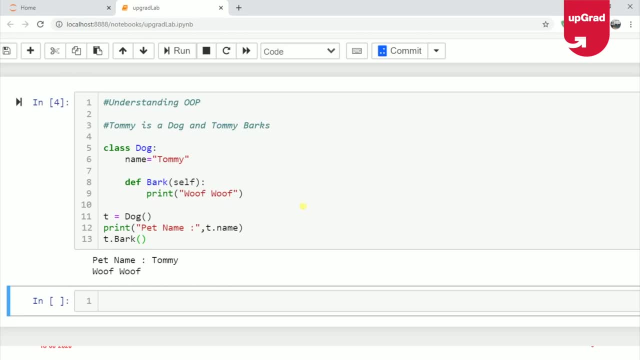 so once again. so what is the objective of this demonstration here? in this demonstration, you must learn how to define a class in python, how to define a variable or a property of a class, how to define the function or behavior, how to create an object in python. how do you access the class? 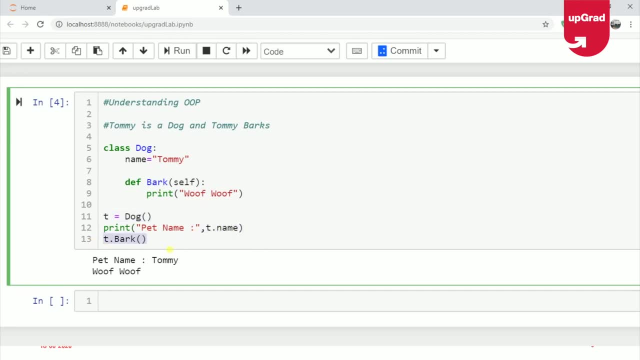 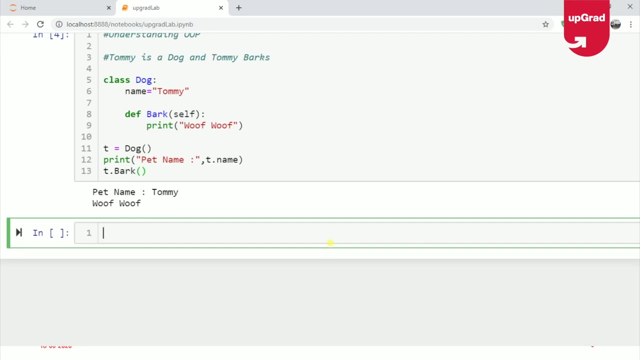 members as well as how do you call the functions or the behavior? so that is the basic understanding of object-oriented programming or it's the implementation of its characteristics, such as classes and objects. let us try to explore more on class and objects using other example. so in this example I'm going to demonstrate you how we can expand or extend the. 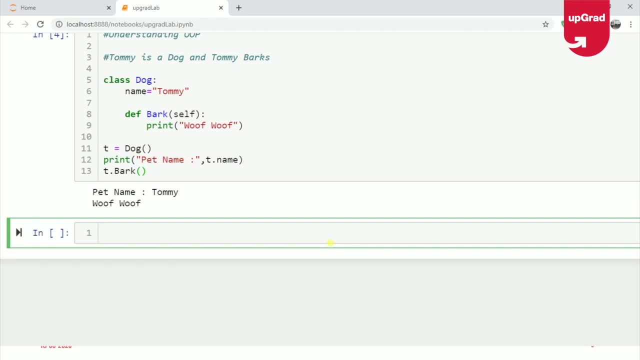 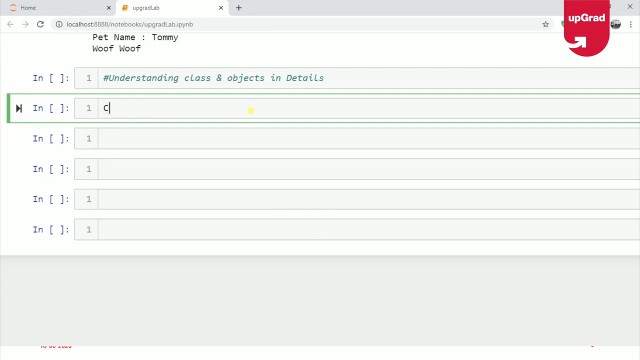 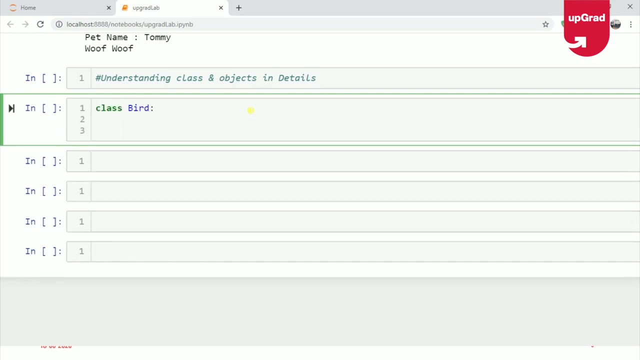 information of an object using some more properties and functions. in this demonstration I'm going to tell you also about the constructors in Python, so let us start with this demonstration. so here I'm creating a class called, let's say, bird. bird has a property called specie. 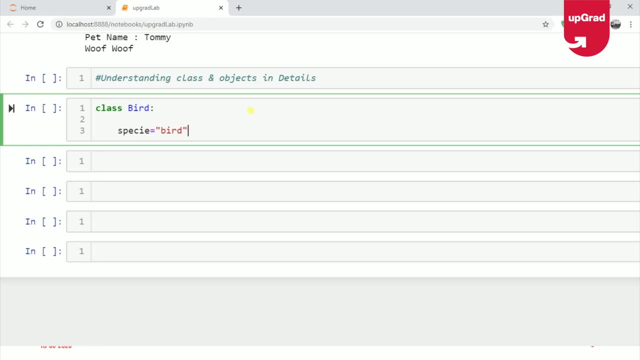 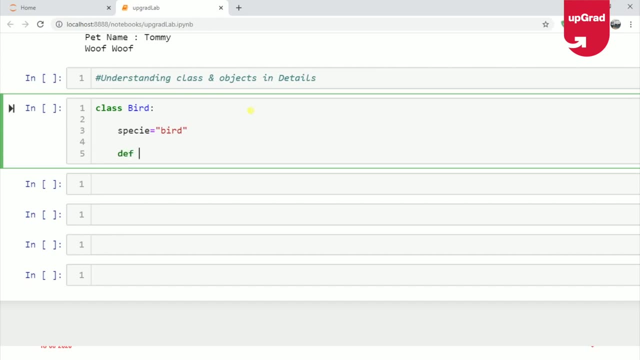 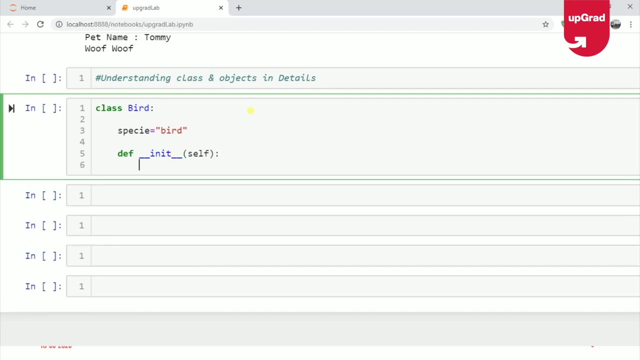 and that is, let's say, bird. now here we have a special function in Python which we call constructors. a constructor is defined using this init syntax here. so first of all, before proceeding, let us understand what is the. what is the purpose of constructor? a constructor is used to allocate memory to the object. 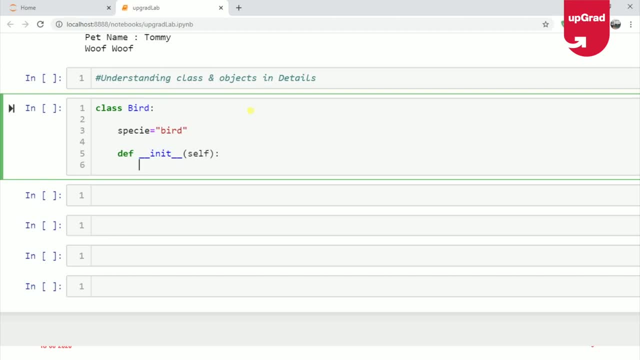 how it allocates memory. we will surely understand that in the next lesson. further, also requesting to please focus on the syntax of creating a constructor here now. constructors are basically used to, you know, set the defaults of an object. so, while creating an object, if you, if you want to set some initial 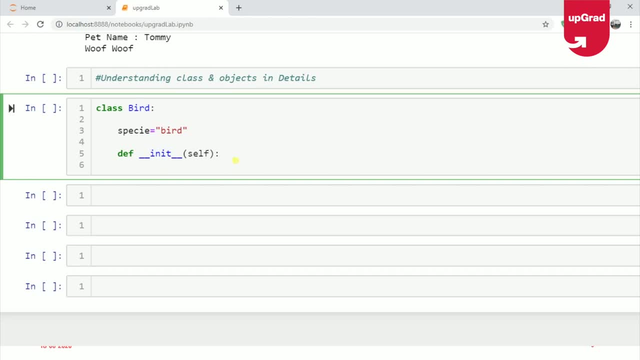 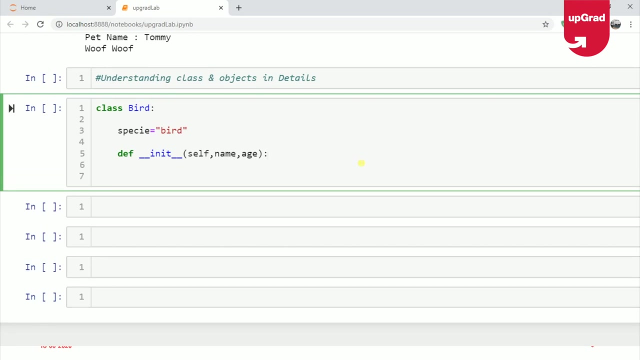 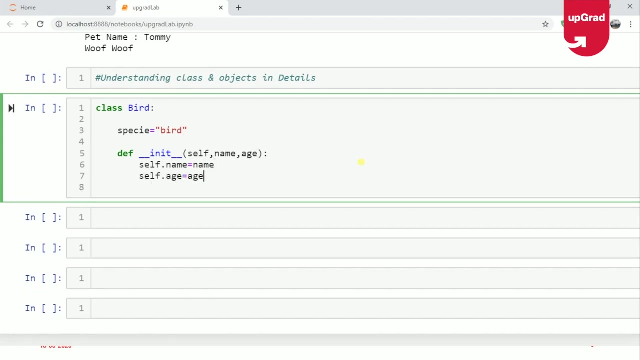 values or initial data for a corresponding object. you can do that, for example, for every bird. I want to set a name and age, so here I'm using constructor for setting the name and age at the time of object creation. so self dot name equals to name, self dot age equals to age. now, what does this? 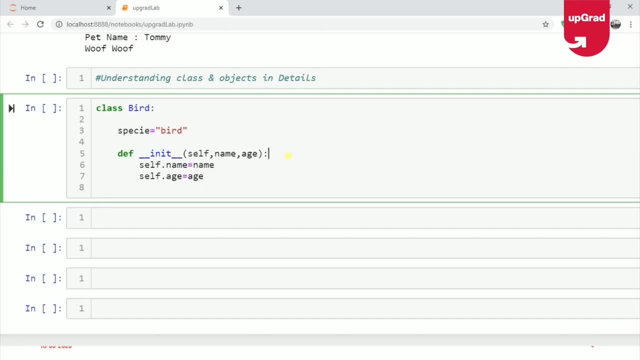 means? this means that any data that I will be passing here will be stored in this name variable. now there is a difference here between this name and this name and this name. so, because I'm using this variable, using the self keyword means this variable will be associated with the object, because here: 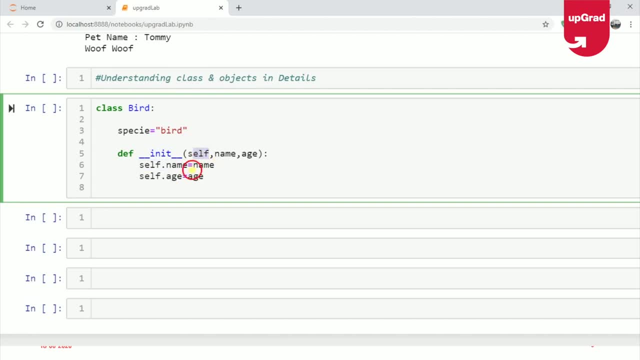 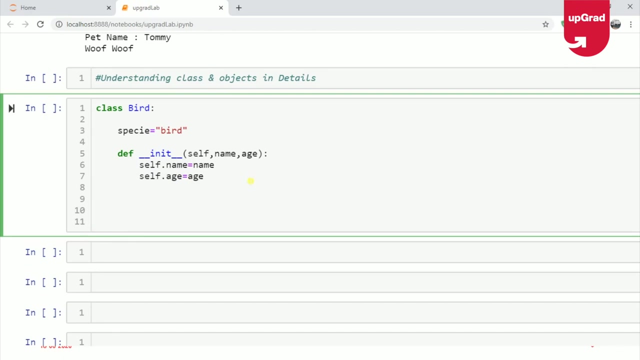 the self keyword or the self word here represents the object. so self dot represents the associative associativity of that variable or the object with with the object of the bird class. now the similar goes with the age variable here as well. So let us try to create an object here. so let's say I'l call it ok, so I'll call it. 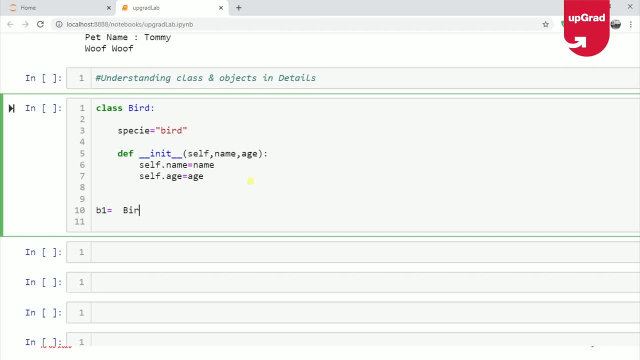 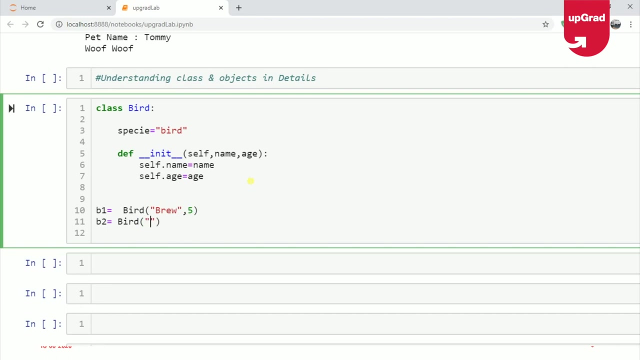 let's say b, one equals to bird Name is, let's say okay. so let's say I Heil Doug brew and I'll call it. let's say five, similarly, b2, bird pico, and let's say two. so here this expression is responsible for the invocation of the constructor, everyone. so this expression will. 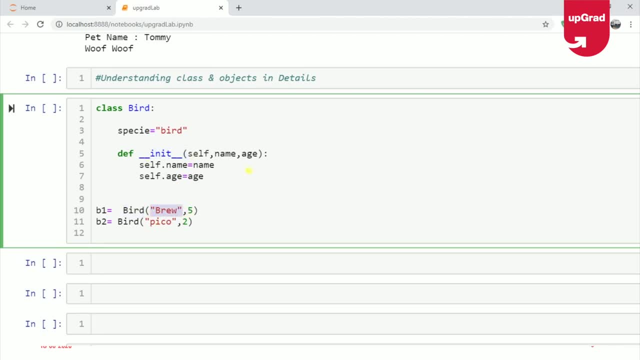 call the constructor and the name of the bird will be stored in name variable here. similarly, the age will be stored in the age variable. now, this data, which is being passed here as the argument to the constructor, will be received here and similarly, one by one. so these variables will be storing the 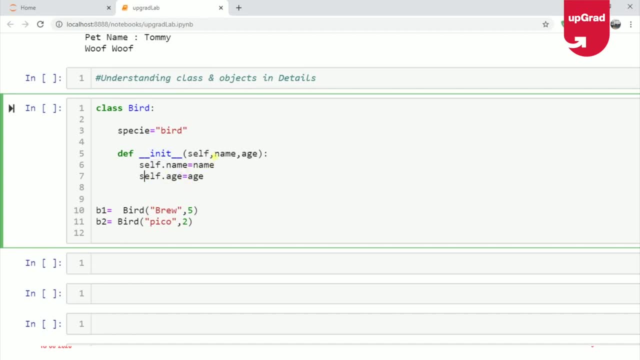 same data. remember, guys, as I told you earlier, self represents the object of the class here. so here the object of the class is b1. so at this line of code, while this code is being executed, this self keyword is is representing the object who is calling this constructor. so in our case it is. 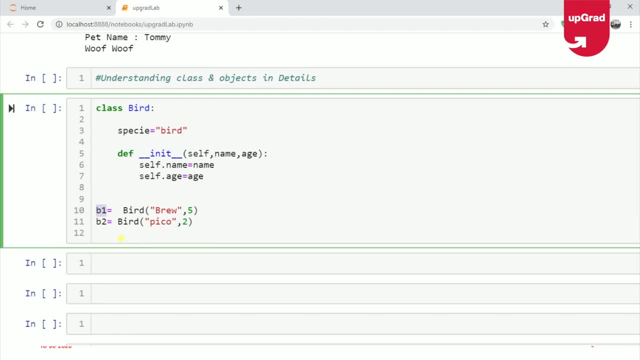 b1. we'll do the same thing with the second object. here, b2 equals to bird. so here this expression is responsible for calling this constructor, and this pico will be getting assigned to name, and two will be getting assigned to age. now, here, once again, this self is representing the object. who is 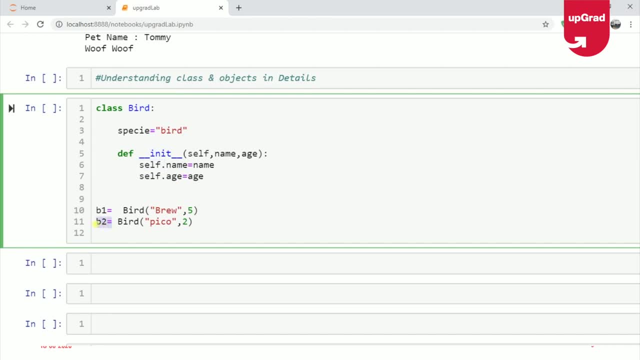 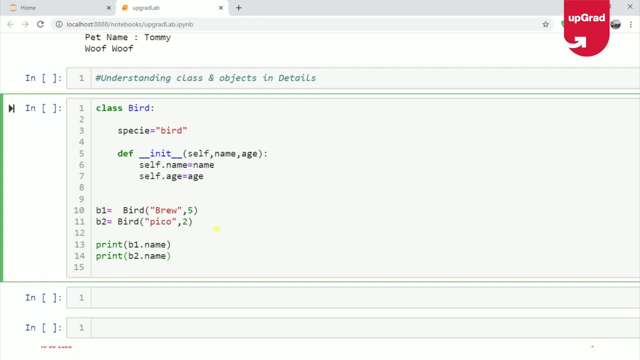 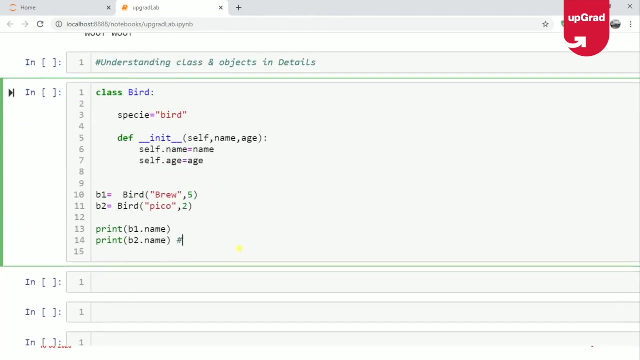 calling the constructor and here is b2, so this name and age gets created and will be associated with this b2. so if I print, let's say, b1 dot name and print b dot name, I get different names here. so I'm using the short key for executing, and that is shift plus enter and the short key for executing. 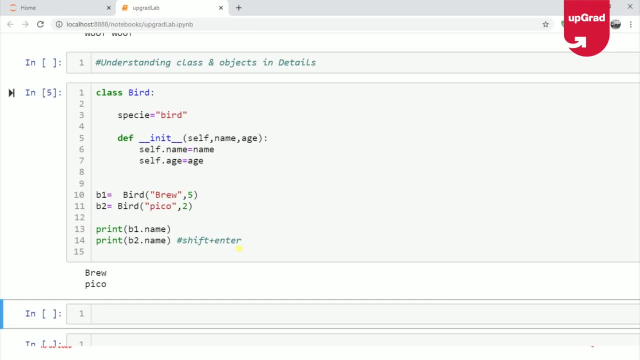 so here you can see that I'm getting different names here: one is brew and one is pico. so here in this example, we expanded our information, or the knowledge, on using class and objects along with constructors, and remember constructors are used for allocating memory to these objects means. 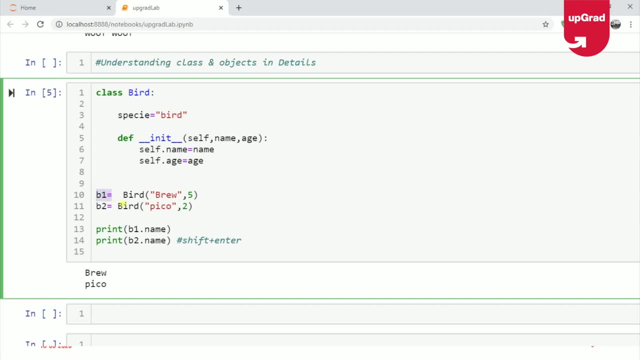 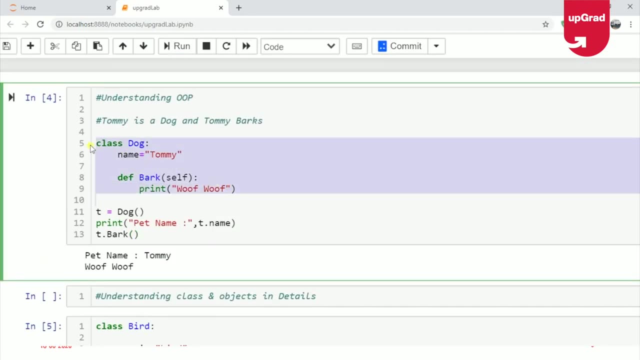 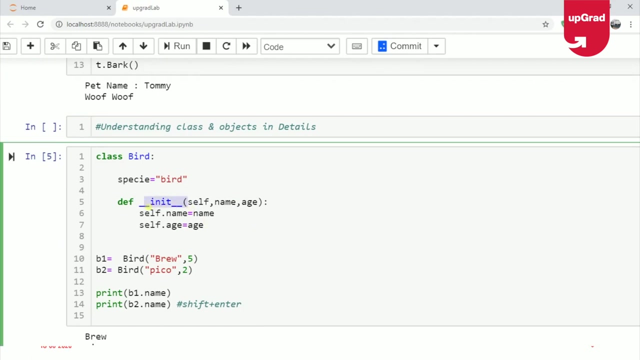 these objects are only created physically, in our system only when these constructors are called. but here in the previous example we have not created any constructor, but still this object was being created. the reason is because, in case, if we do not define any constructor, the python compiler will create the constructor for 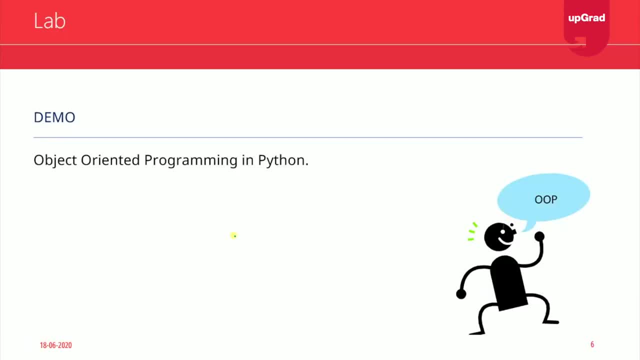 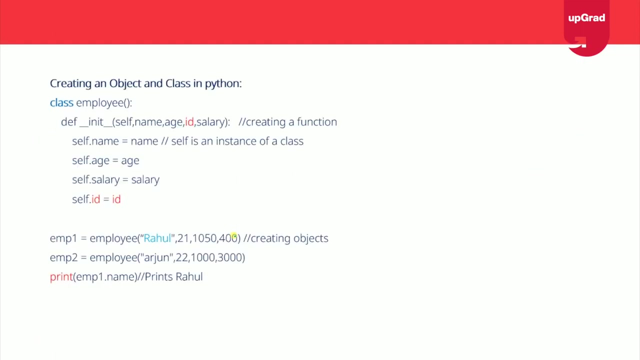 us. so with that practical implementation of classes and objects in python, I'm sure that you have understood clearly how to implement the characteristics of object-oriented programming, such as classes and objects in python. so here is a demonstration of class here. so here, in this example, I'm trying to explain the similar things here: how you can create a class, how you can. 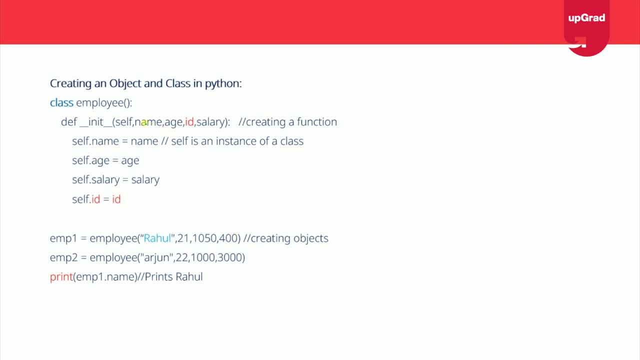 create a constructor here, how you can, you know, set some default parameters here, default properties here, and how you can associate the data with the objects here. so in this example you can see that i'm creating the object emp1 for the employee class, with some default values here. similarly, there is one more object called emp2, with some. 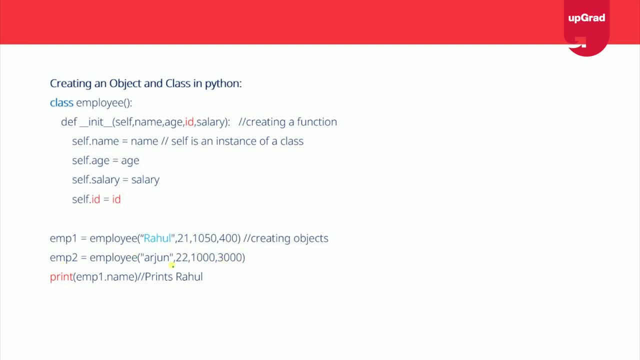 different data here which is getting assigned, which is getting associated with emp2 using the help of the constructor. here i'm accessing the value or the property of a emp object, emp1 object. all right, with that, let us start and let us try to explore some more interesting and exciting. 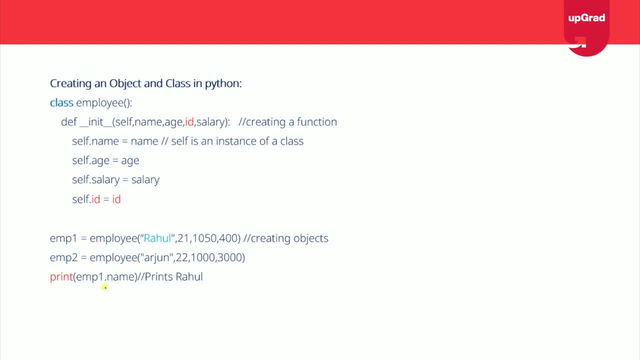 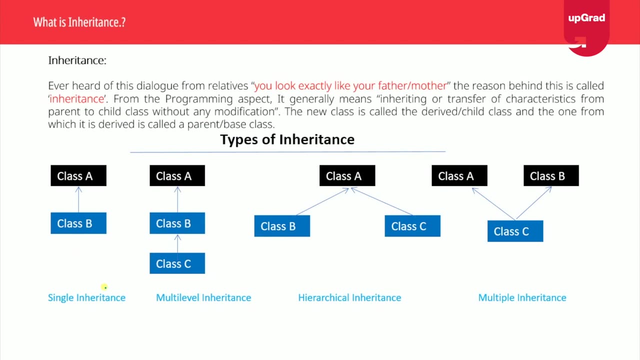 concepts of oop or object-oriented programming in python, and that is inheritance. so you might be wondering: what is inheritance? you must have heard of a popular dialogue from your relatives that you look exactly like your father or mother. now what does that mean? that means that where we 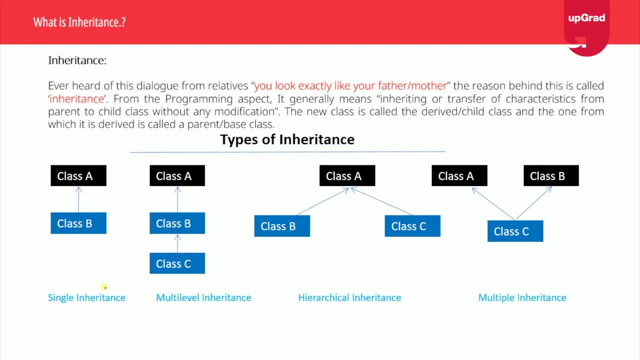 we derive certain characteristics or properties from our parents. now, when you, when you, acquire certain properties or behavior from your parents, that acquisition of properties or behavior is called inheritance. so so inheritance generally means inheriting or transferring the characteristics from parent to child. let us try to understand the 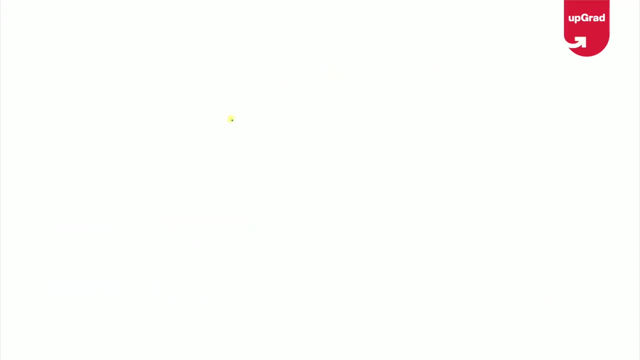 inheritance and inheritance, careful understanding of inheritance andили we are not sure if inheritance inheritance. with an example here. so let's say there is a class called vehicle and you know that there are certain properties of vehicle here, such as the price of the vehicle and the dimensions of the vehicle, and you can. 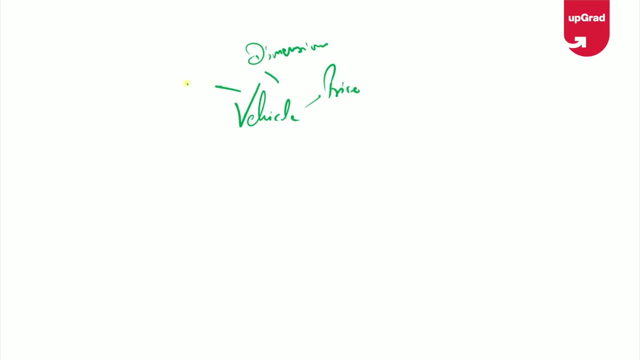 call. let's say, for every vehicle there will be a fuel type, so whether it is petrol or diesel or any other. now here we have other class called car, and car inherits or acquires its properties for vehicle. so if car acquires its properties for vehicle, then car will automatically have these properties, such as fuel type. 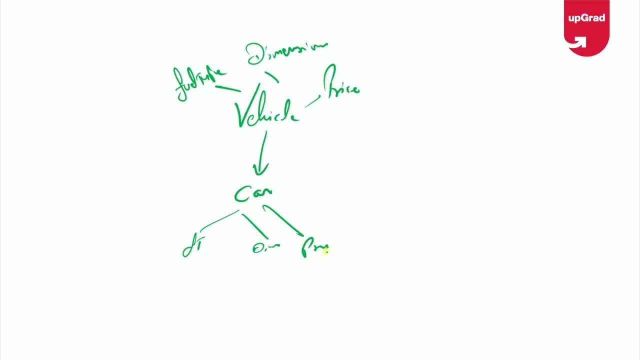 dimensions and price. so this acquisition of properties or functions from one time to next time, or a number of times, will be bola superposition. it shows all these properties here. so our class to another class is defined as inheritance. now, when we learn inheritance, it is important for all of us to understand some terms here that we use. 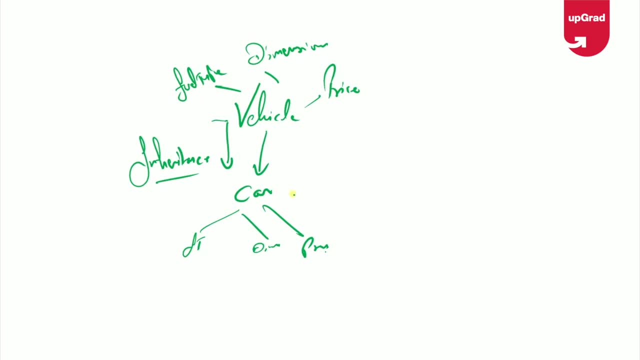 while implementing inheritance. and that is what is a derived class. a derived class is a class which receives the properties from other class so that this class is called derived. so this class is called base class. a base class is the provider class: a provider class which provides the properties and functions to 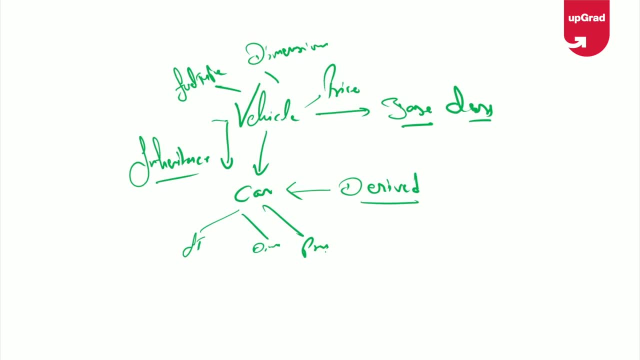 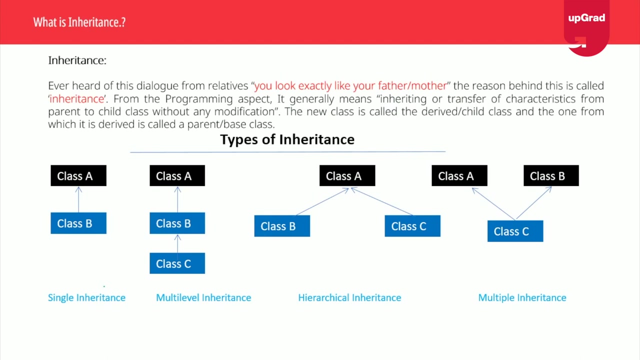 any other class. so here it is important for all of us to understand the base class and the derived class terminology. now, with that, I hope the inheritance is clear to you, and now let us try to understand the different types of inheritance that we can implement in Python. now, the very first type of inheritance in Python is single. 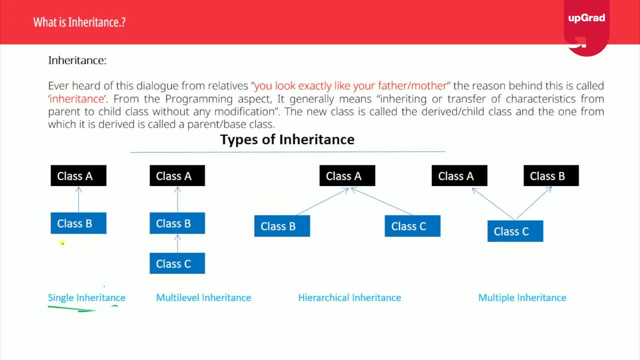 inheritance. it's a very basic and general type of inheritance in Python. so what does it means? it means that there will be a class, let's say B, and it will be inheriting its properties or acquiring the properties from it, so it's like 1 to 1. second is multi-level inheritance. so in this multi-level 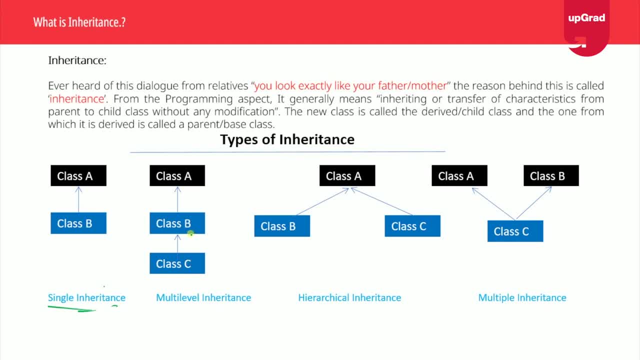 inheritance: C is properties from B. B is acquiring properties from A. So here C will indirectly get the properties of A. So this is multi-level inheritance. This is hierarchical inheritance. In hierarchical inheritance we have two different classes, let's say B and C, and they are acquiring the properties. 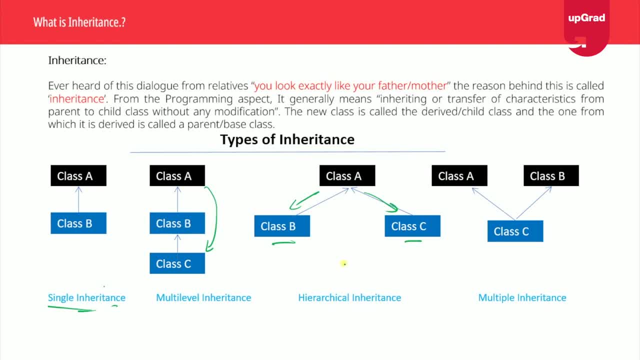 from the class A. Then we have multiple inheritance. In case of multiple inheritance, a single class acquires the properties from multiple classes, such as here. in this example, class C is inheriting or acquiring the properties from class A and class B, both. Let us try to. 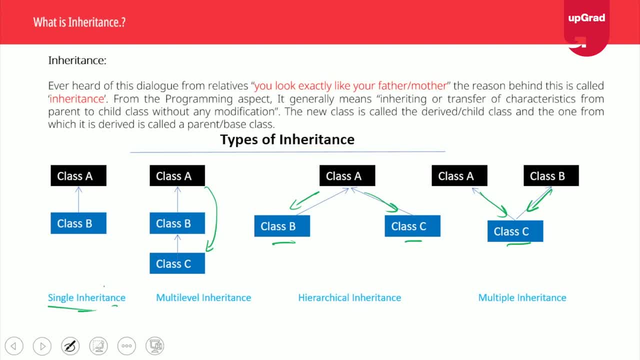 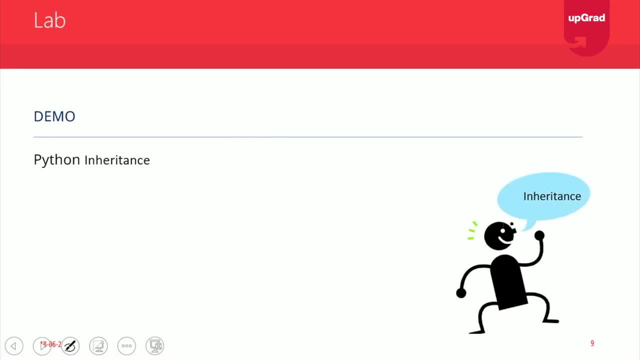 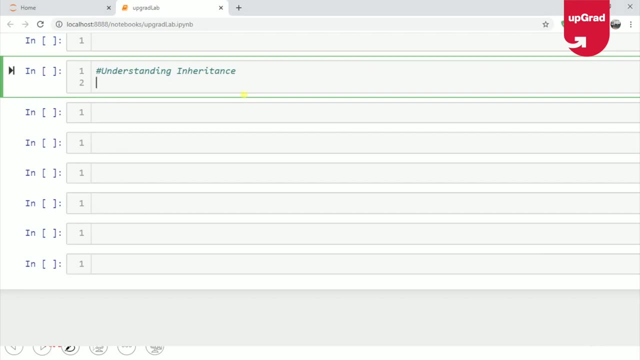 understand- this is, these types of inheritance- by doing some of the practicals here, Let us start In. So here, the very first type of inheritance that we are understanding here is single inheritance. Now, single inheritance is pretty easy to understand, So let us implement it this way. So 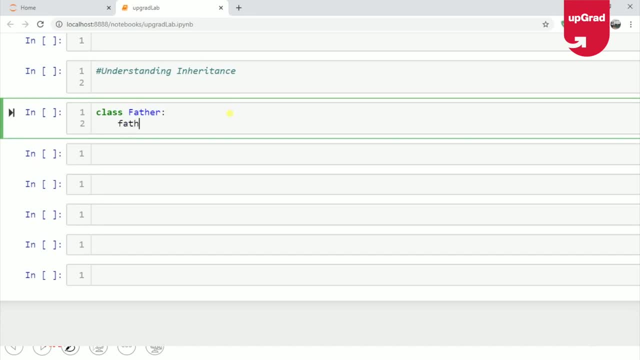 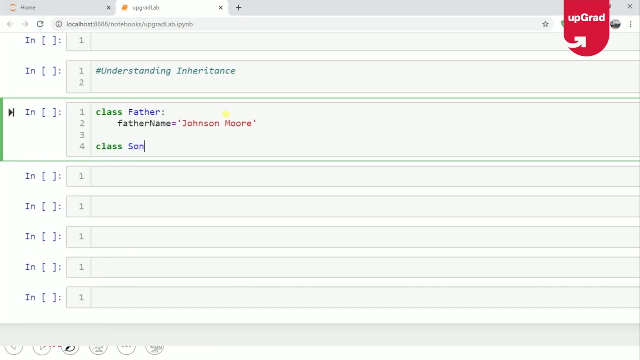 here we have a class called father and here is a property called father name. Now here we have another class called son here, and this is the syntax of inheriting from any other class. So please observe the syntax of inheriting a class here. So here father is the base class and son is the 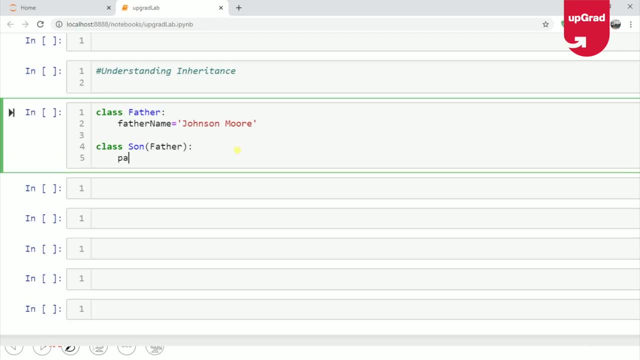 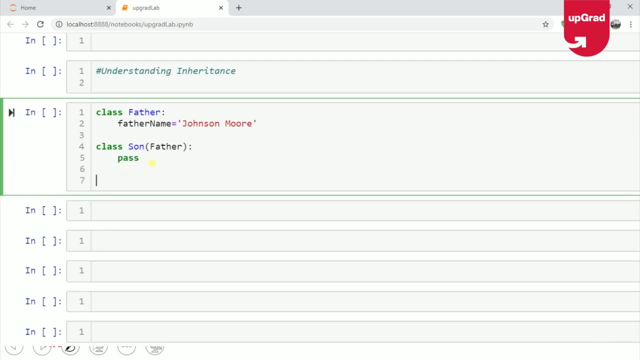 derived class. So I'm just keeping the class empty here. So that's why I'm using a keyword called parse here. So let's say, if I create an object of the son class, Okay, Let's get rid of the in the middle class. So I'm going to create the in the middle class, And if I 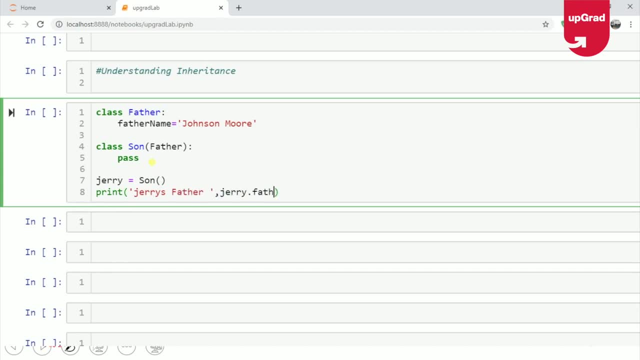 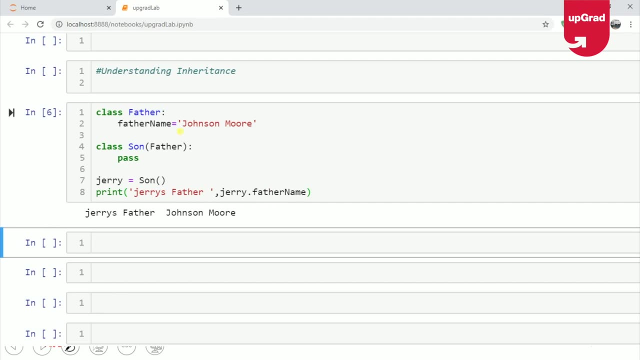 print Jerry's father, Jerry dot father name. So here you can see that in this example I'm able to access the property called father name using the object of the son class, Although here we can see that there is no variable or the property- father named- defined in the son class. 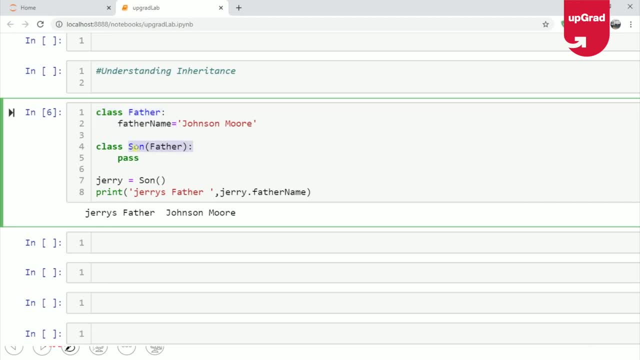 this class. here the reason is because of inheritance, because this inheritance make makes this variable available to us in this sunglass. let us try to check this and let us try to remove the inheritance here and here. I'm going to execute this demonstration once again, and I must get an error here that you 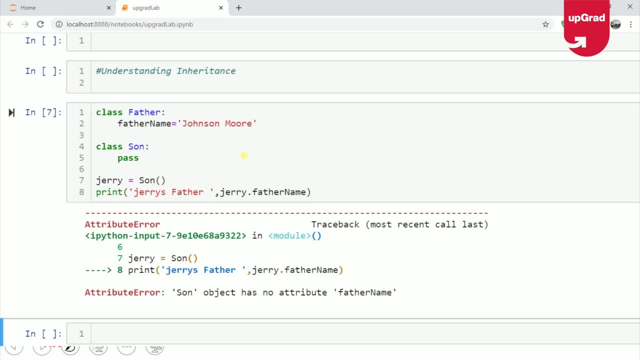 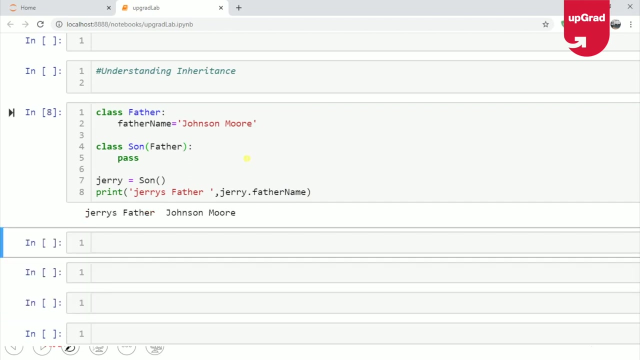 can see here. the reason is because this time we don't, we do not have implemented the inheritance here and son is not having any access to father name. let's correct it to its back previous state, and here it is. so this is an example of a single inheritance, where one class inherits from the different class. so 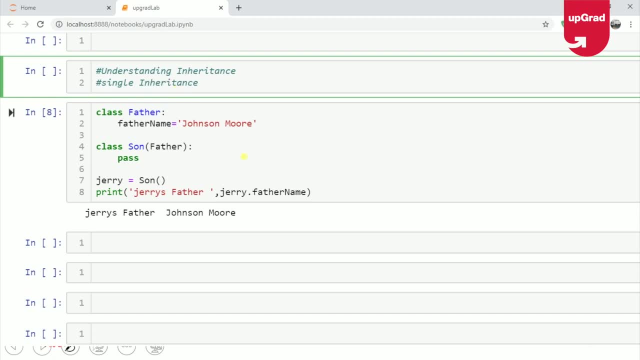 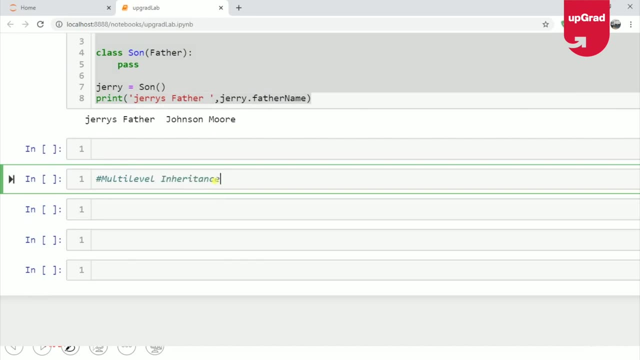 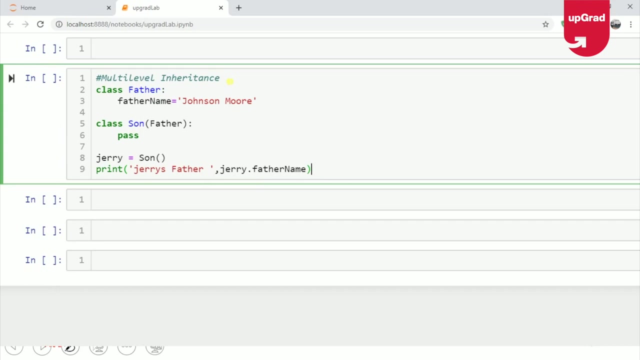 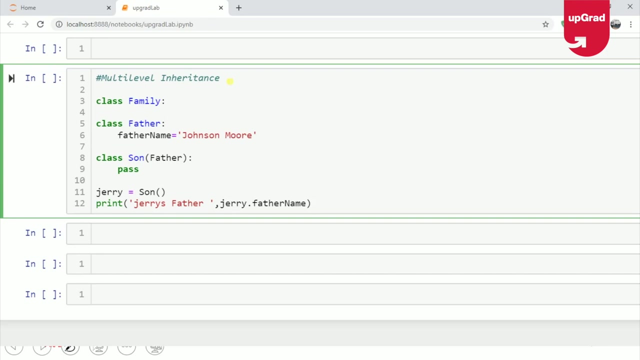 this was single inheritance. now let us try to understand multi-level inheritance- inheritance in Python. so, in order to understand what is multi-level inheritance in Python, let us create one more class here called family. so there's a class here called family with a variable called origin. and let's say: 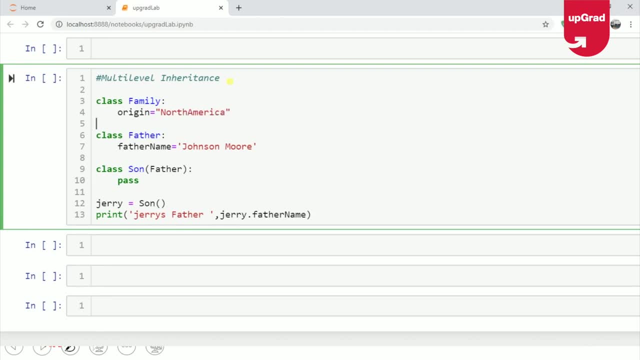 North America. here you can see that father inherits from family, so let us try to understand the inheritance of father, and father inherits from family, so let us try to understand the inheritance of father and father here here. so here is the family class. so Thank You. regarding the polarity and 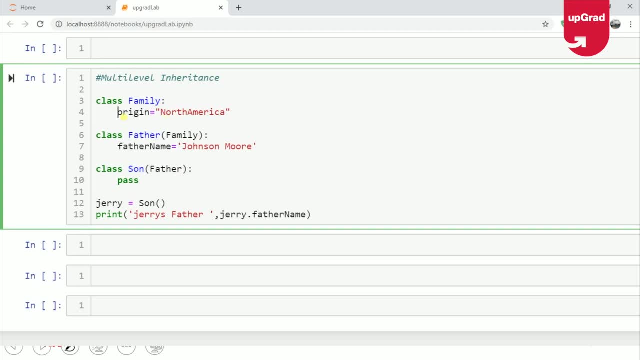 the family class. so in order to understand the family class bound hierarchy here. so son inherits from father, father inherits from family and it's the family class. the family has a property called origin here. so this must be available in father now, because I am inheriting father here. so this results in the acquisition of the origin variable from the family into the. So this is what a family can content from parent to son life there and I am testing the family attorneys for animal, which I ambonizing father by recently because, Michael, let us try and let's test it. let us try, and how is it working? I am tuned to M1, so what have you been doing online for the así? if you want to download the driver, nicely, pre-cal FARTA strategy is you have to get all the information. now the� try. and what have you been doing online for burial problems? now, these are all these. 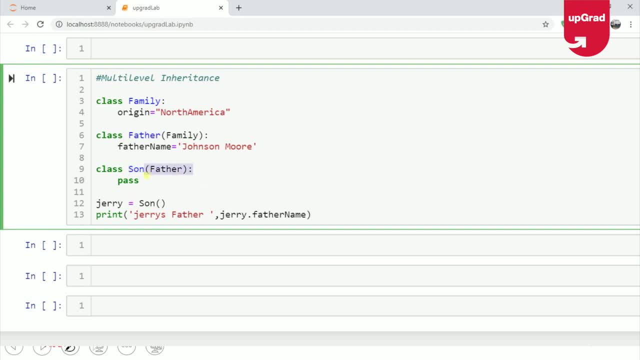 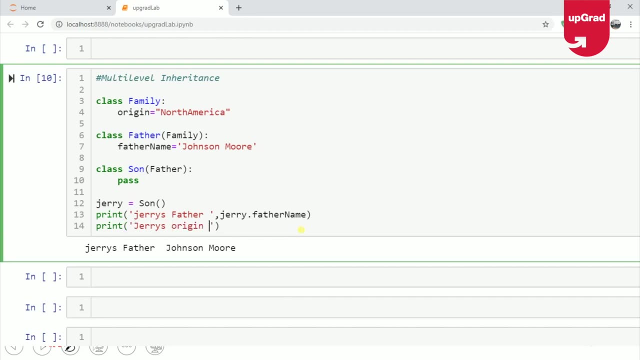 tested whether we can access the origin from some, so we'll print origin. so here you can see that I'm accessing in the property not from its base class but from the class which this its base class inherits. so if I execute this demonstration, you can see here that it prints Jerry's origin: North America. so 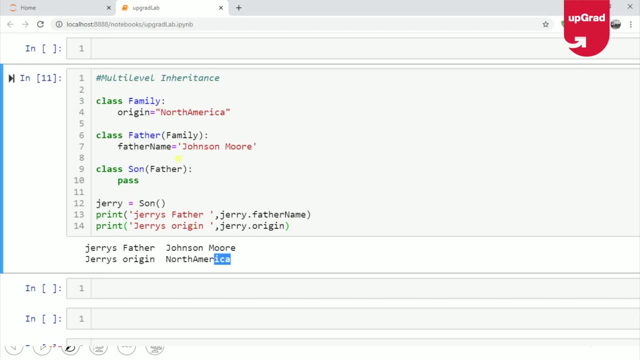 here we must understand the implementation of inheritance here, where family is being inherited by father and father is being is being inherited by son there by result, resulting in the availability of the family in the derived class here. so this is called multi-level inheritance. now let us try. 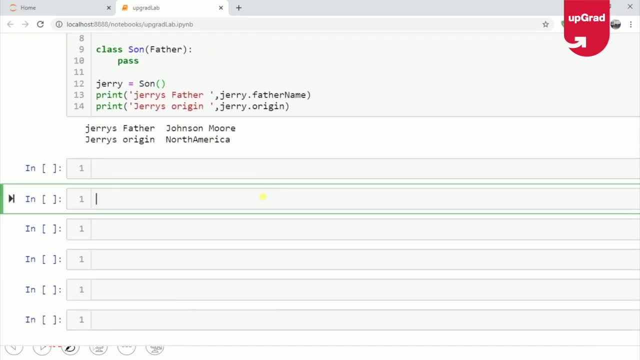 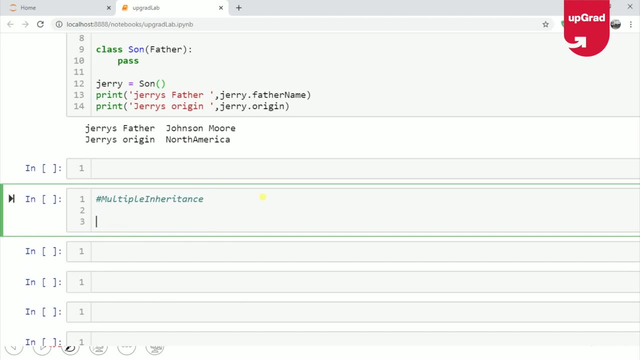 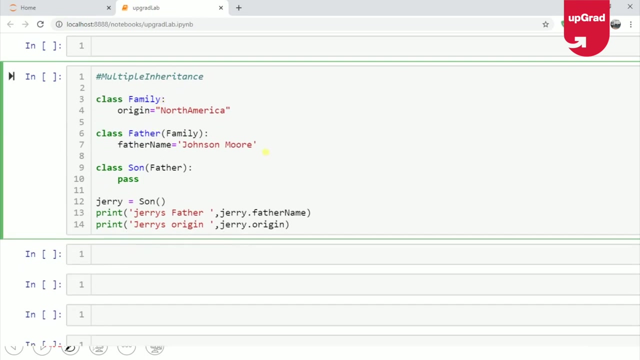 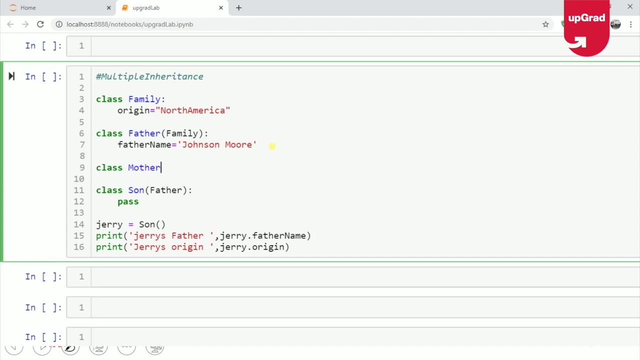 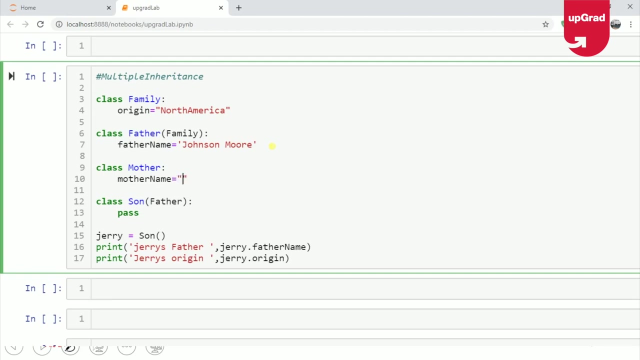 to understand one more type of inheritance here, and that is multiple inheritance. so in order to understand multiple inheritance in Python, let's create one more class here, and that will be mother. so here mother has got a variable. call it, say, mother name, Susan. so here I have added one more class called mother. now, in order to 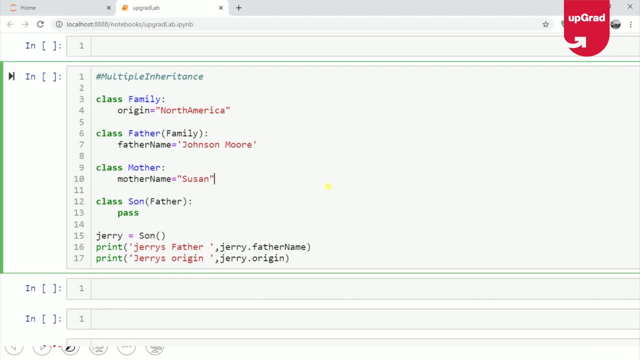 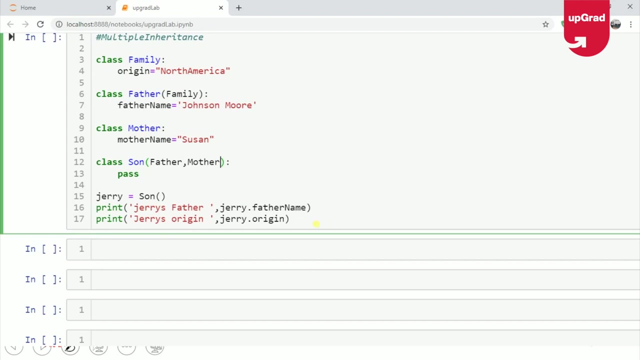 implement multiple inheritance. a single class must inherit from multiple classes. so here, in this case, son will be inheriting from father and mother both. so with this inheritance here you can see that son must have access to the father name and the mother name variable. here let us try to test it by: 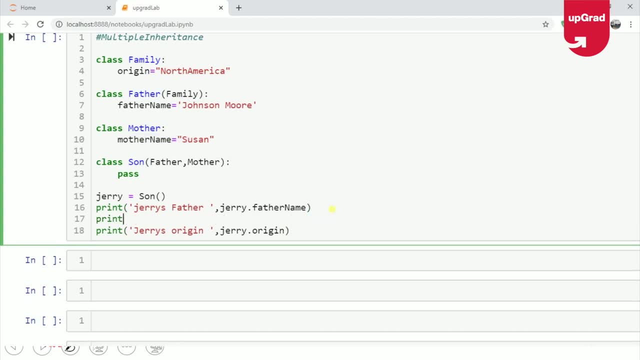 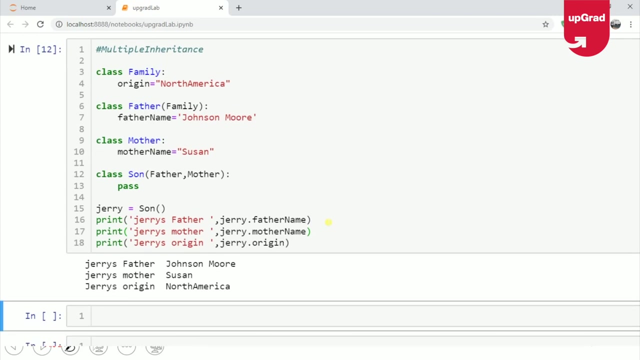 printing the mother name. print Jerry's mother, Jerry dot mother name. let us execute the demonstration and let's see if it works. so here you can see that Jerry is able to access the properties from father as well as mother. so this is an example of multi-level integration. 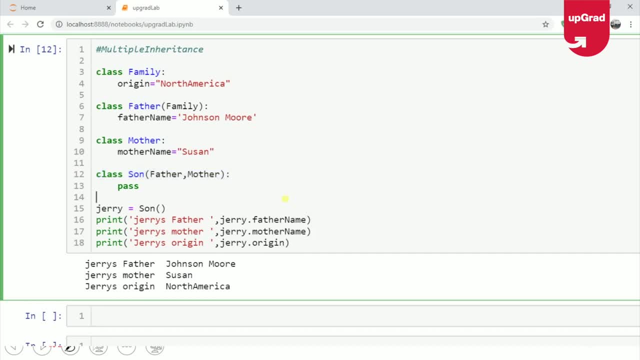 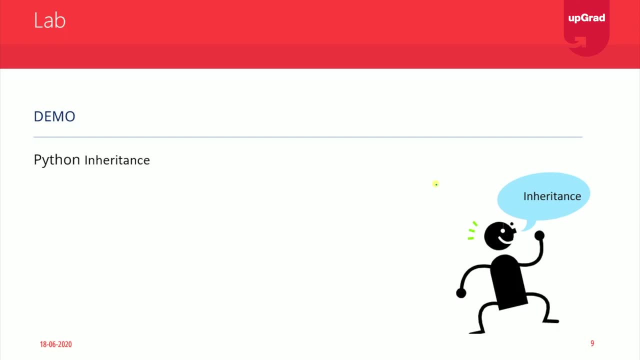 multiple inheritance in Python. so that was the implementation of inheritance in Python. I hope you have clearly understood what is inheritance and their various types. so we discussed some of the types of inheritance here, such as multi-level, multiple and single inheritance. that must give you a clear understanding of how to implement inheritance in Python and the various 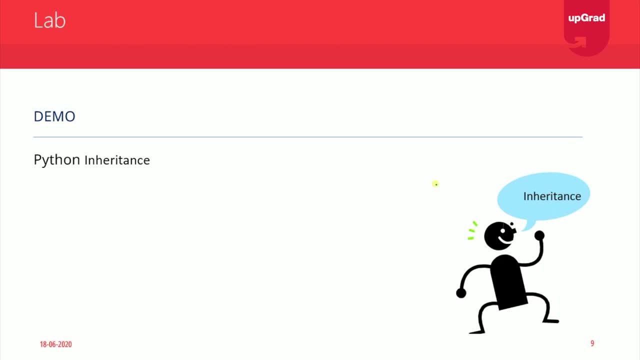 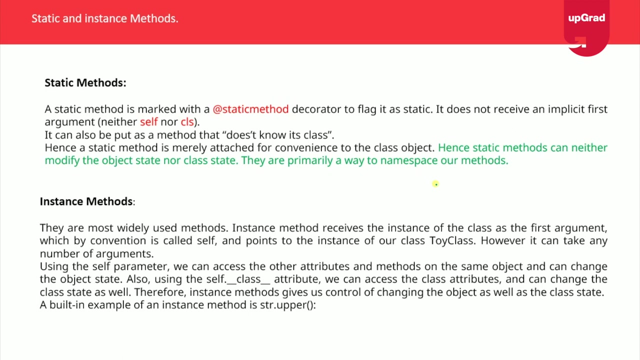 terminologies associated with it. now let us try to understand one of the most important concepts of object-oriented programming, and that is differentiating between static and instance methods. now, static methods and instance methods are the most integral part of object-oriented programming because they might change the behavior of your code, so it becomes critically important for all of us to 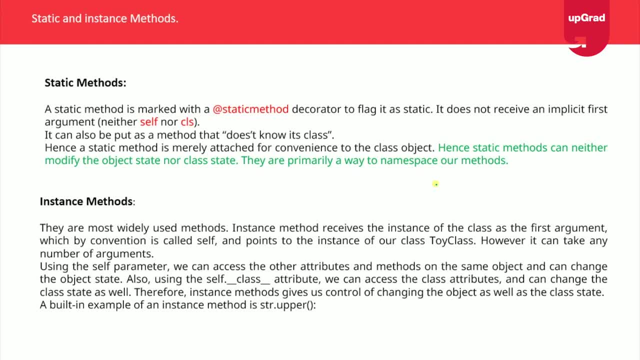 understand what a static method is now. methods in Python are extremely similar to Python class level methods. The difference between a static method is that it is bounded to a class rather than the object. So what does it mean? basically, It means that you know, we can. 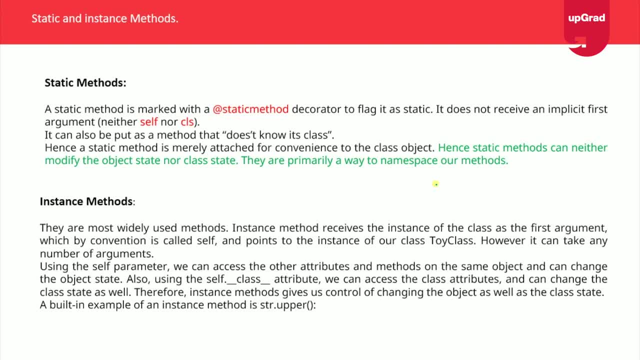 call the static methods without need of an object here. So this also means that the static methods cannot modify the state of an object. that's true, The static methods. the reason for not being able to modify the state of an object using static methods is because static methods are not associated with the 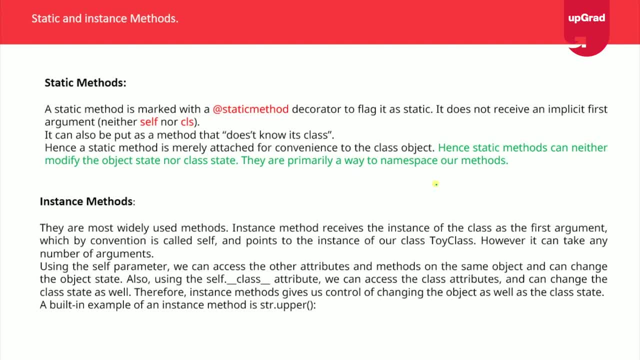 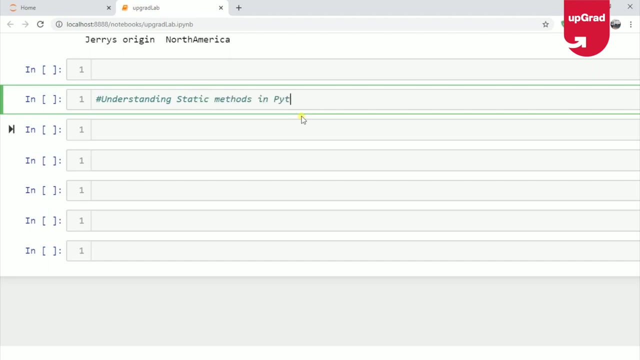 objects. they are bound to the class. So let us see a programming demonstration and let us try to understand how to define a static method and how does they work. Then we'll be discussing about the instance method as well. All right, understanding static methods in Python. So, in order to understand, 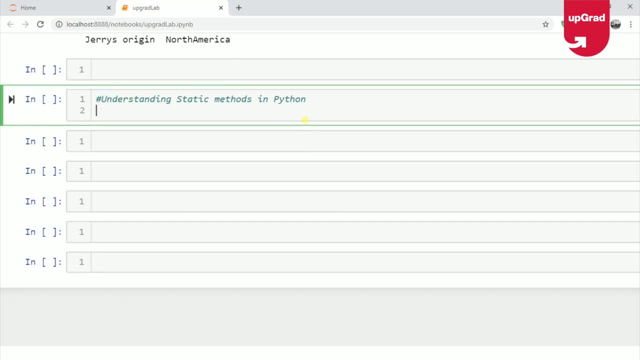 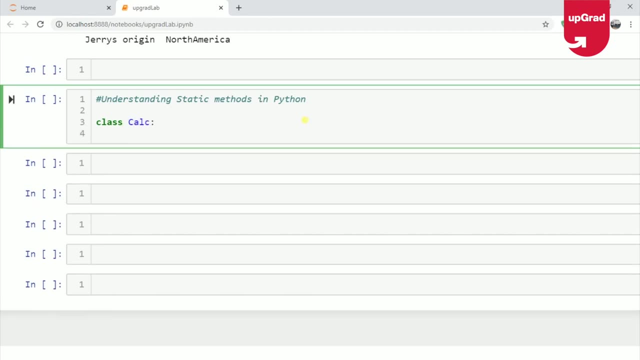 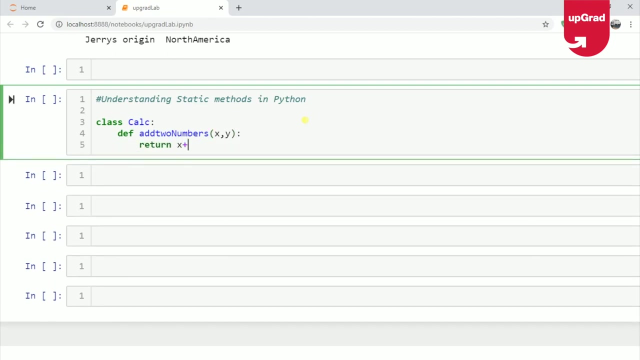 static methods in Python. let us try to create a demonstration here. So here we have a class called calc and here we'll be defining a function. def: add two numbers: x comma y, return x comma y. So here, first of all, the very first thing that I wanted to. 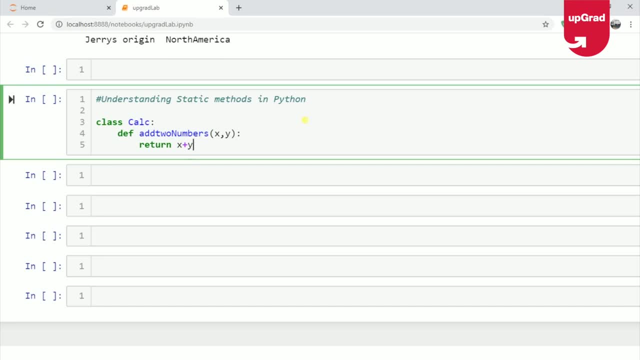 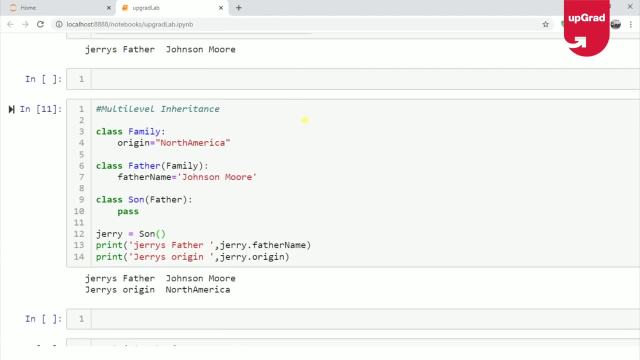 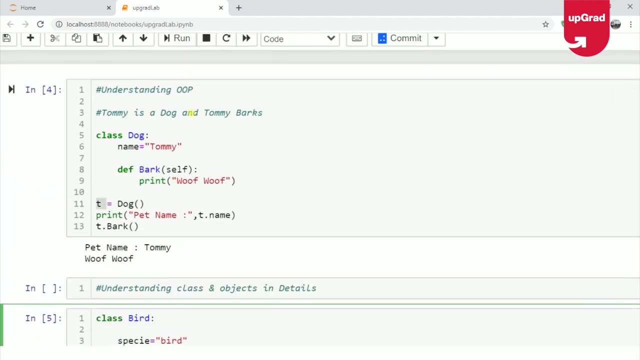 observe is that in this method, add two numbers. I am not adding the self keyword. If you remember the previous examples, in the previous examples I used to add a parameter called self while defining a function in a class. So I can show you here as well. you can see the self parameter Now, this self keyword. 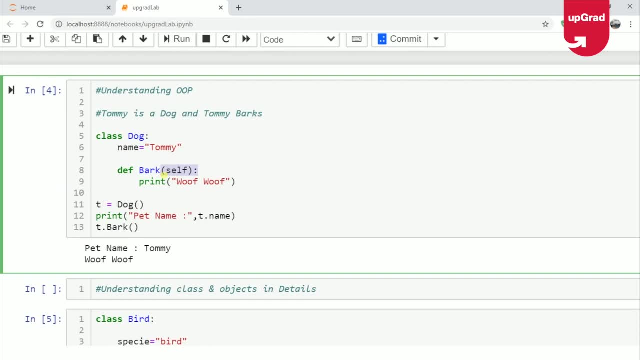 represents the object here, which clearly indicates that this is the function of the class. so we can see the self parameter now. this self keyword represents the object here, which clearly indicates that it is in the class that this function is basically associated with the object here. Now the 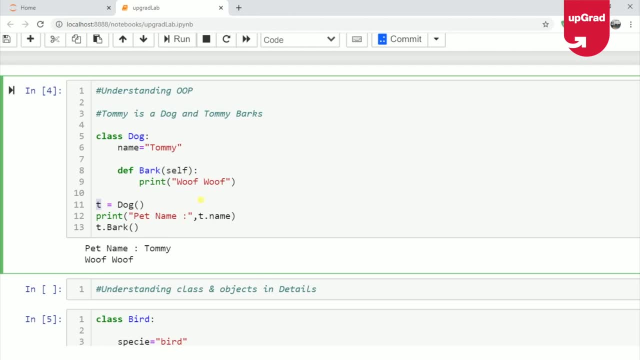 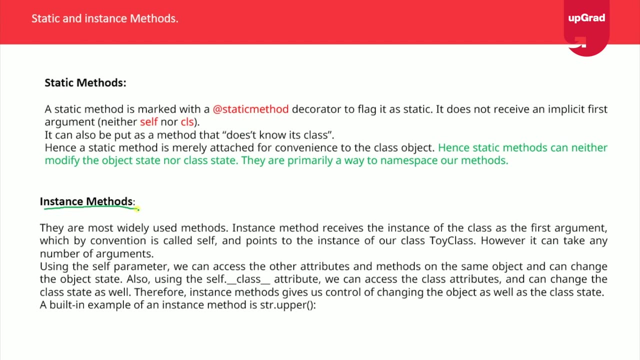 functions which are associated with the objects are also called instance methods. So here instance methods are basically those methods which are defined with the self parameter and represents or indicates its associativity with the objects. Instance methods are also able to change the state of an object because they are associated with the objects, But that is not the case. 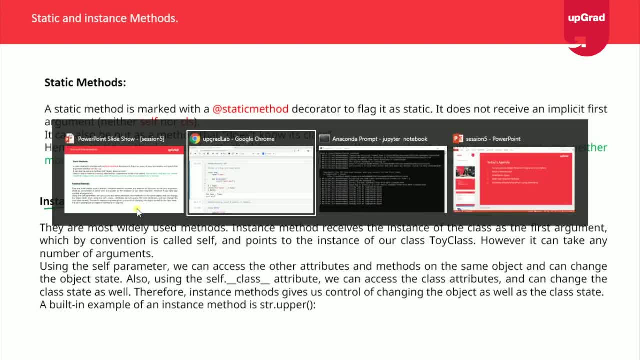 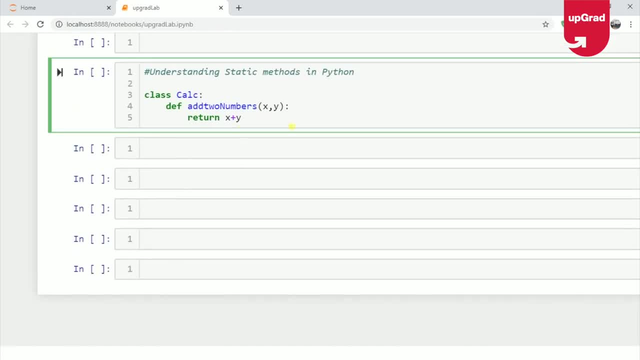 with static methods. They are completely different and are not bounded with the objects. So let us proceed further and let us extend this demonstration here. So in this demonstration, we are trying to understand how to implement the static methods. Once again, the very first difference that is to be observed here is exclusion of the self parameter. 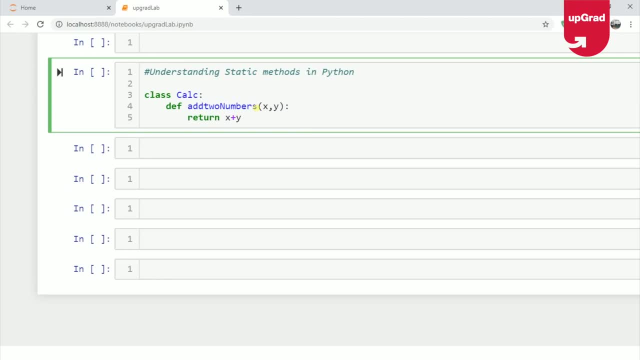 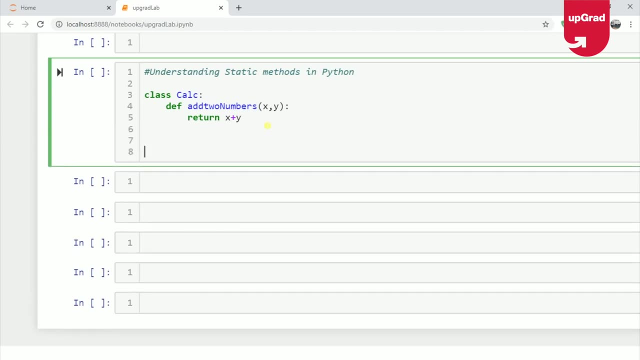 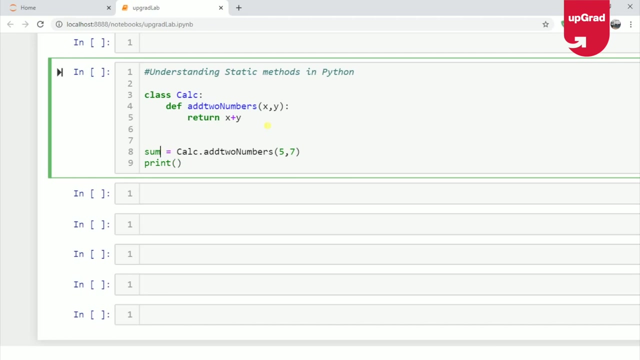 here. Alright, so how we'll be using this function in that case? So here, observe the expression here. So let's say sum equals to calc dot. add two numbers, 5, and let's say 7.. Print sum 1.. So here, in this example, if you observe that I have not created any object or 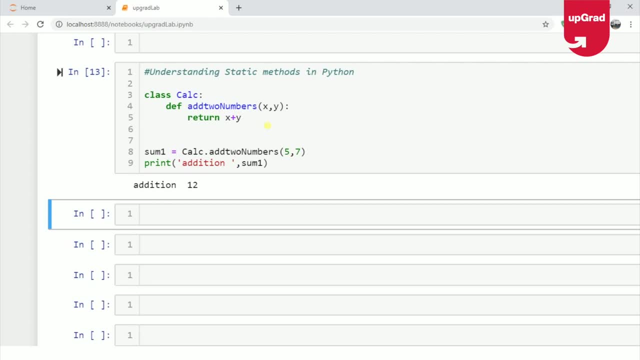 instance of the class called calc, and without the need of the object or without creating the object. here I'm accessing the function using the class name. Now here, because this function is a static function or a static member, so that's the reason I can access this function using class name directly. So here I am called a static function, so that's the 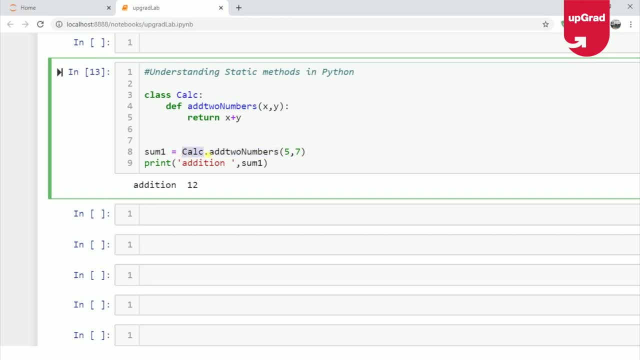 reason I can access this function using class name directly. So here I'm calling a static member. So that's the reason: I can access this function using class name directly. So here I am calling a static function, otherwise this thing is called hanging norms and 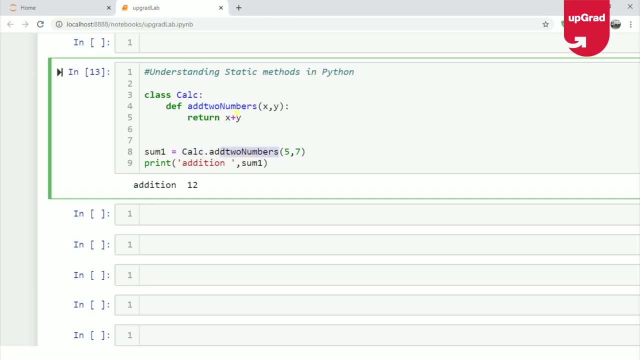 So here I'm calling the addToNumbers, which is here passing 5 and 7 to the corresponding x and y variable, here, which returns me the sum here goes inside the sum1, and it creates the sum. So this is a very basic understanding of how to define a starting method in Python. 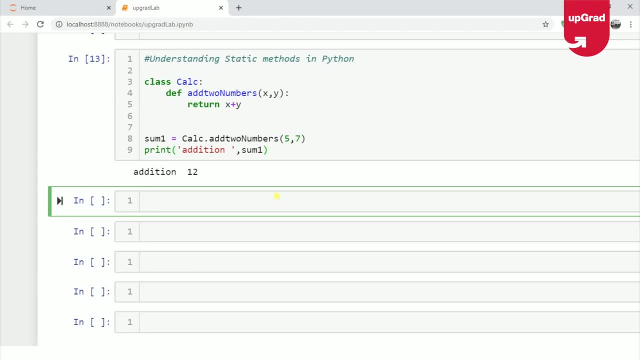 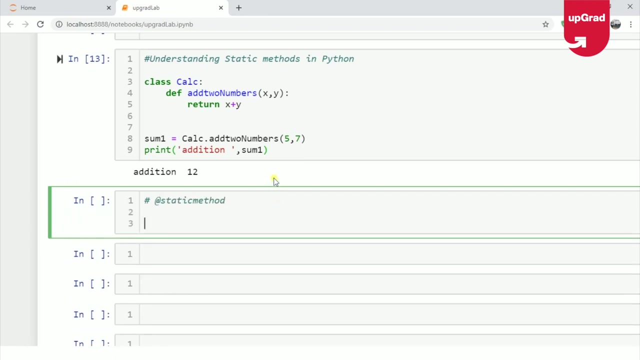 Let us try to understand the different approach of implementing starting methods in Python. So here I'm going to use an annotation, here called at the rate static method. So let us try to understand how to use this annotation for creating starting methods in Python. 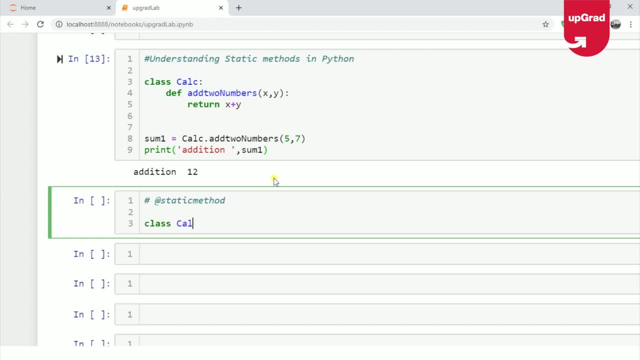 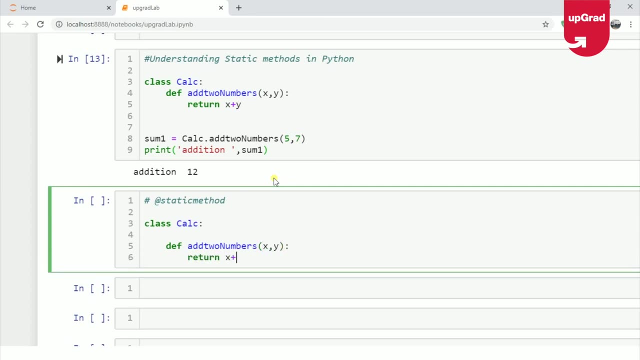 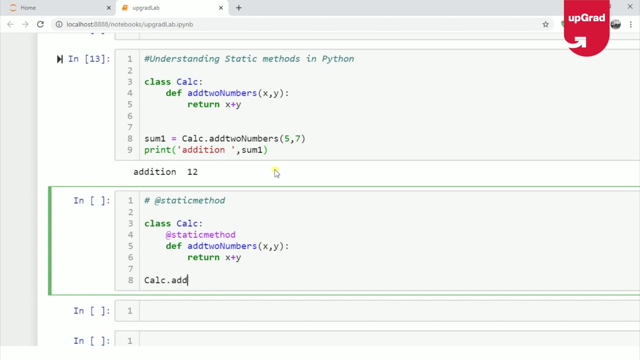 We'll follow the same approach here. class calc, def, addToNumbers x and y, which returns x plus y. But this time what we'll do here, we'll mark it with an annotation, here called static method. Now, the advantage of marking a method using starting method annotation is that every time 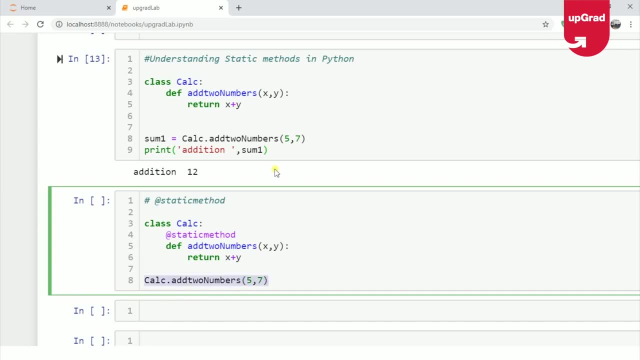 we do not have to rely on this expression to define the function as static Now, but when we access a function using class name, That's only when the function will be treated as a starting method in Python. But here, using this annotation, if we mark any function as a static method, then the 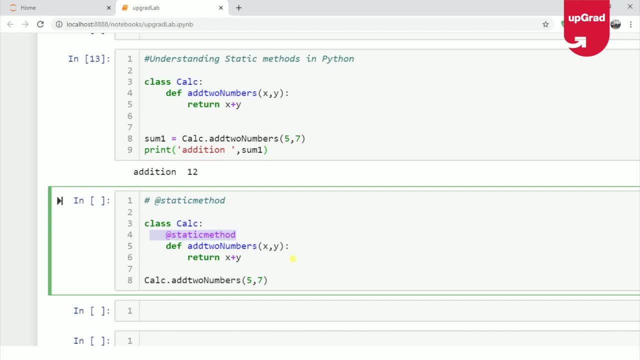 compiler will be previously aware of the function behavior and its outcome. So here the starting method marks a function as a static at the compile time only, instead of runtime. Now if we print it we'll get the same output. So that was the other approach or other method of implementing starting methods in 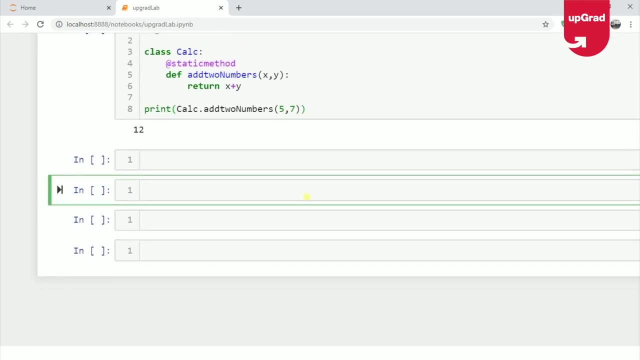 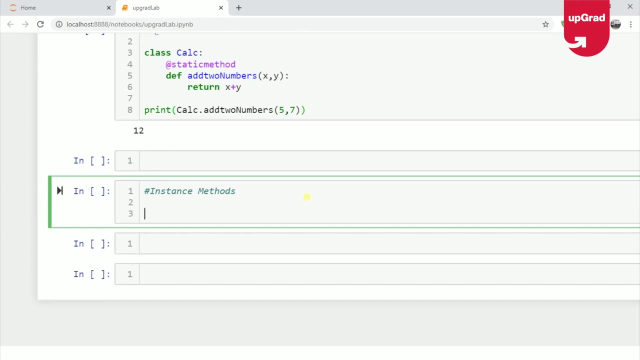 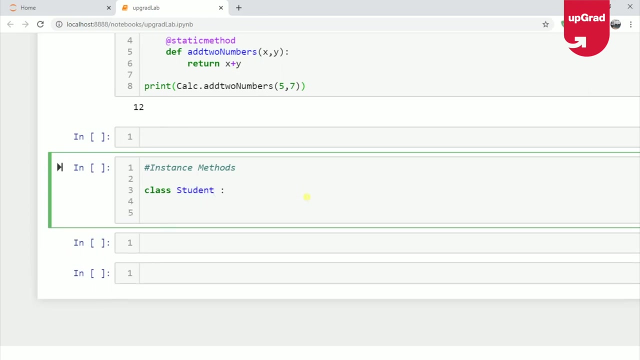 Python. Now let us try to understand the instance methods here. For understanding instance methods, let us try to create an example here of student. All right, So here we'll call a function called, let's say, set marks Mark. 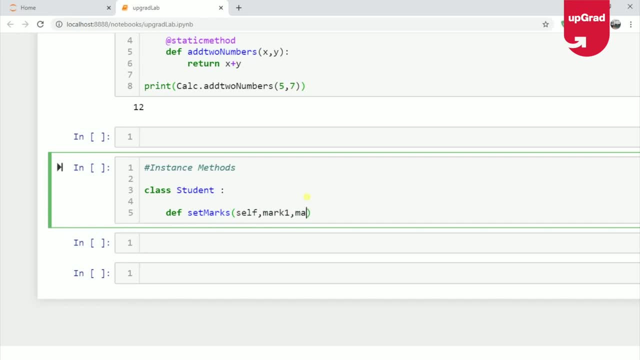 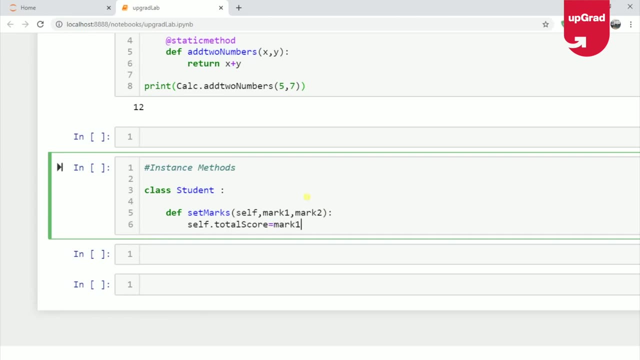 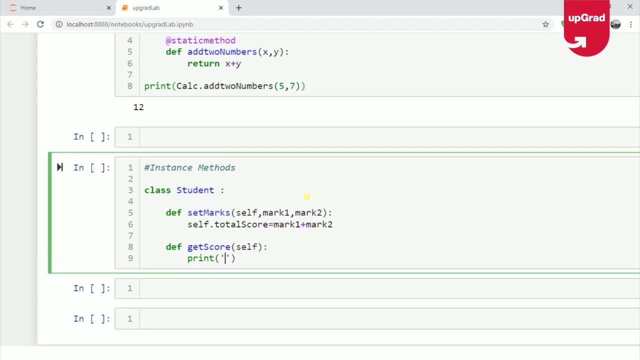 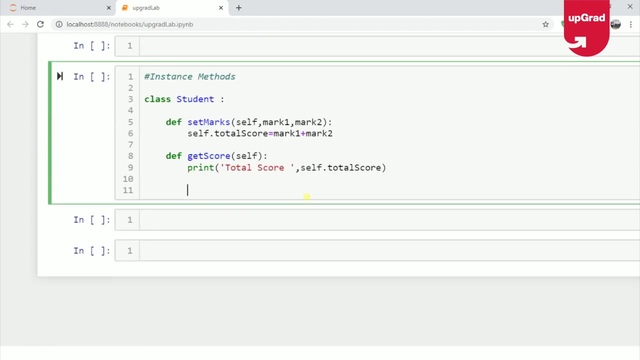 Mark1. Mark2.. selftotalScore equals to mark1 plus mark2.. def. getScore self print totalScore comma- selftotalScore. So here you can see that in this example I'm using the self keyword here, which represents the object. 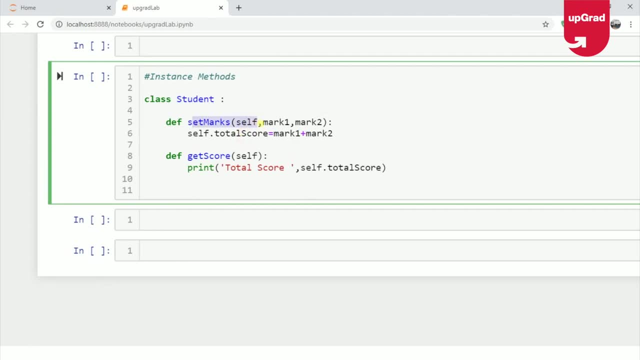 Now This really shows that this object and the variables defined inside it are associated with the object, which can also modify the property of objects. So here there is one more instance function called getScore, And what it returns? it returns the total score. here. 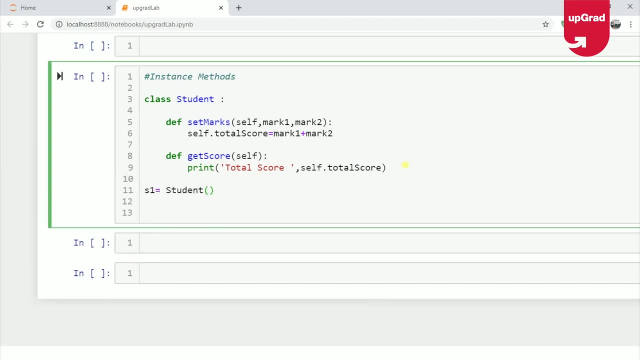 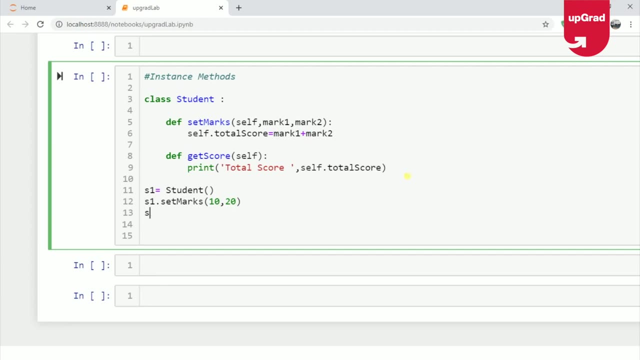 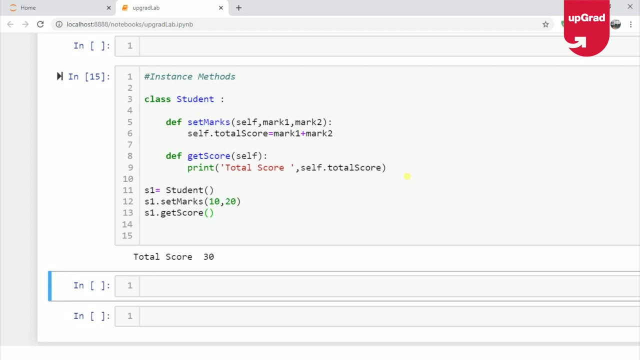 So here, if I say, let's say student and S1 dot set marks 10 and 20.. S1 dot getScore. So you can see here that it prints total score 30. Now what instance methods can do is instance methods can change the state of an object. 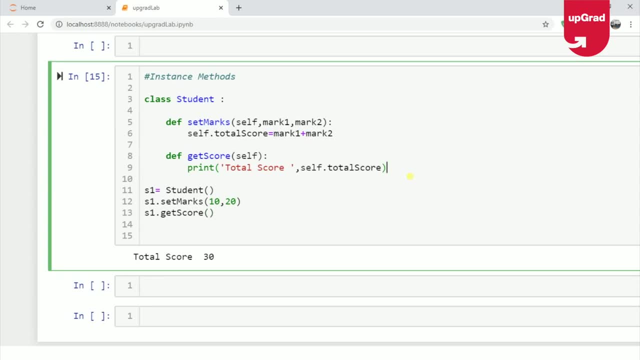 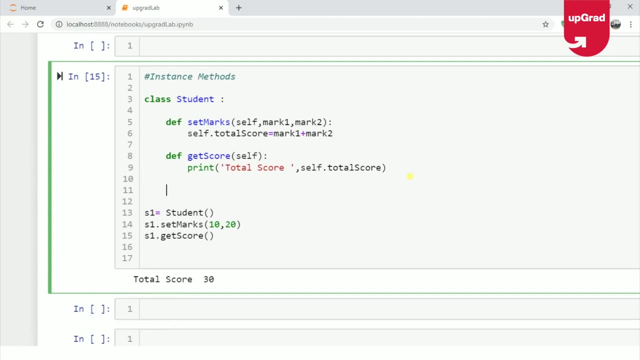 here Now how instance method can change the state of an object is OK. let us look at this example here to understand how the instance methods can change the state of an object. So: def, changeScore, selftotalScore. OK, That's it. 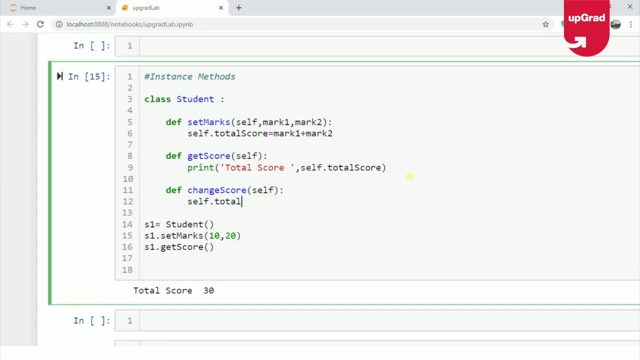 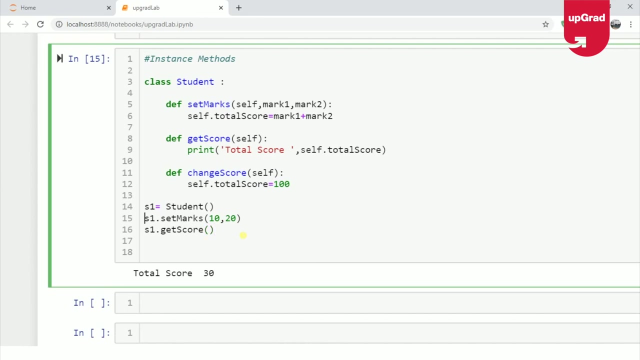 Thank you. And now it's showing S1 dot selftotalScore equals 100.. Now here you can see that I'm able to modify the value of this variable from 30 to 100. here Let us try Setting the score here. 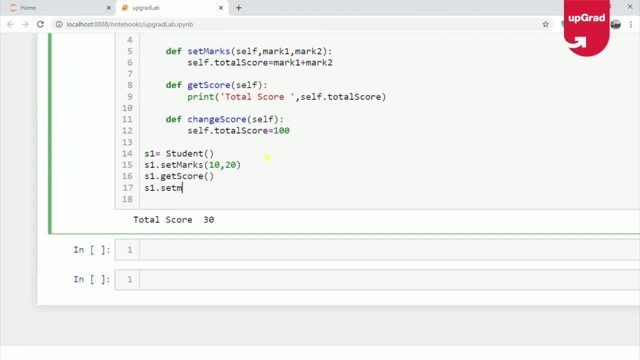 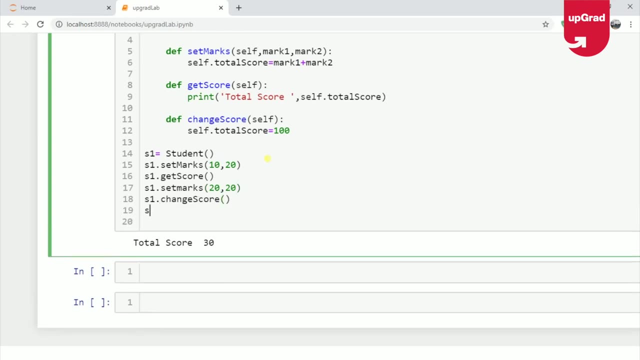 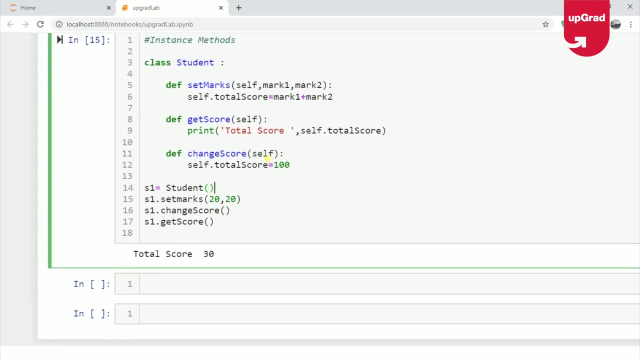 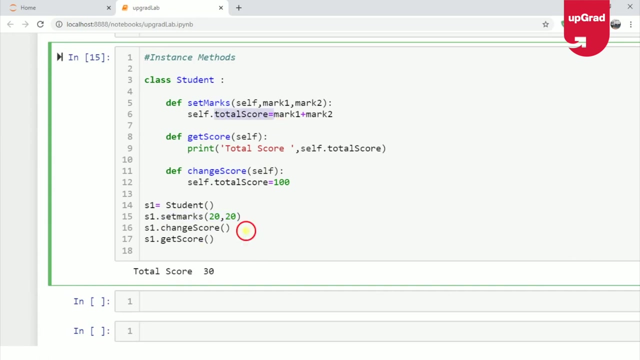 S1 dot set marks 20,20.. s1 dot change score. s1 dot get score. so here you can see that I'm. I have set the marks as 20 and 20, which must result in 40, but before I'm printing the marks by: 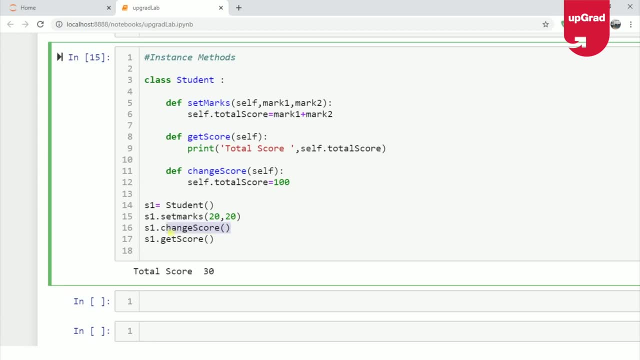 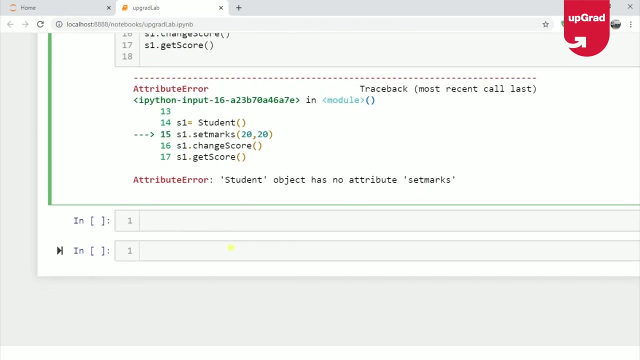 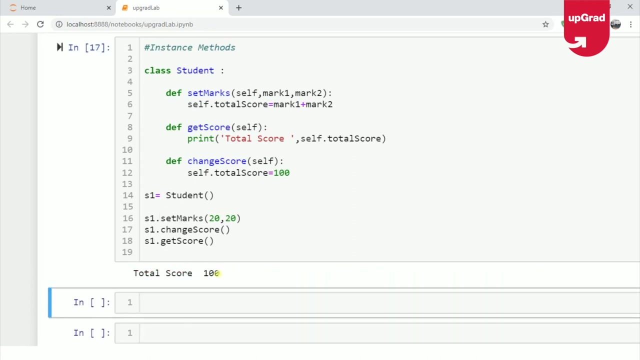 calling the get score. I'm calling change score here now, if you observe all right, set marks, okay. so there is a trouble here. just give me a moment set marks. so here M is capital and here M is small. all right, so let's correct this error. so here you can see that instead of getting 40, I'm getting 100 here. so this: 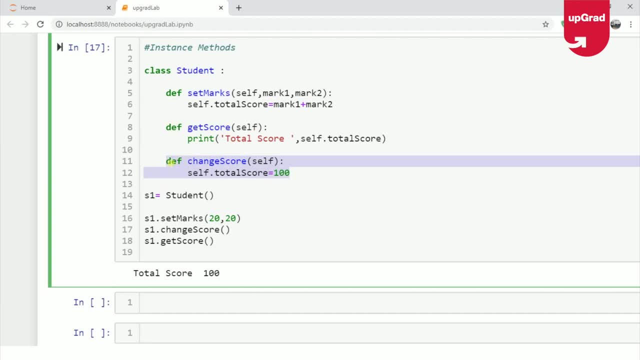 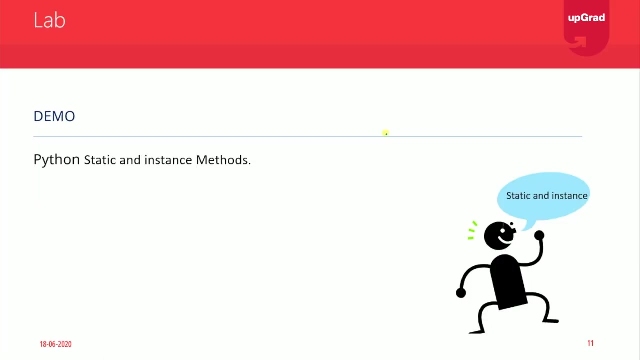 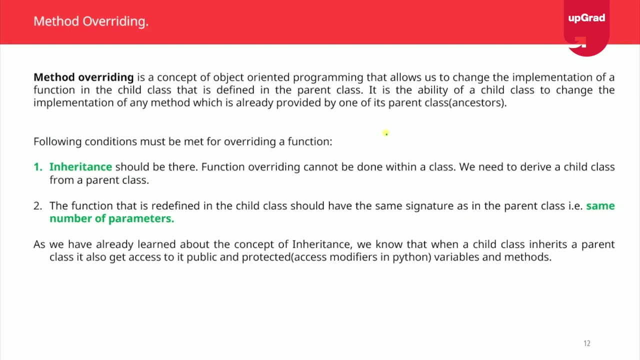 clearly confirms us that any instance function can change the property or the behavior of the object, which is not possible with the static methods. I hope that gives a clear understanding of what is a difference between static methods and the instance methods. with that let us proceed further to the new exciting topic of Python, and that is polymorphism. so here methods of overriding is a. 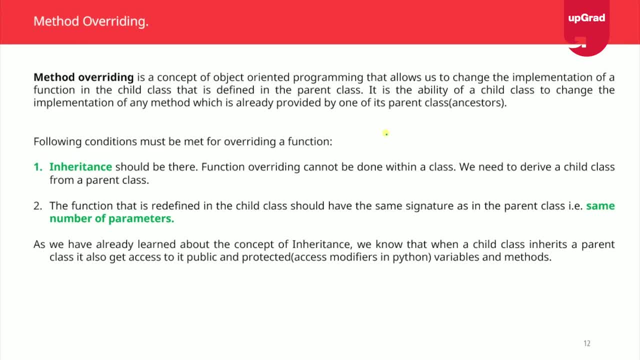 is an example of polymorphism here. so what is polymorphism? first of all, now, polymorphism is an ob, is a, is a characteristics of oop, which basically means that if any object can represent itself in different form, then it holds the capability or it shows the capability of 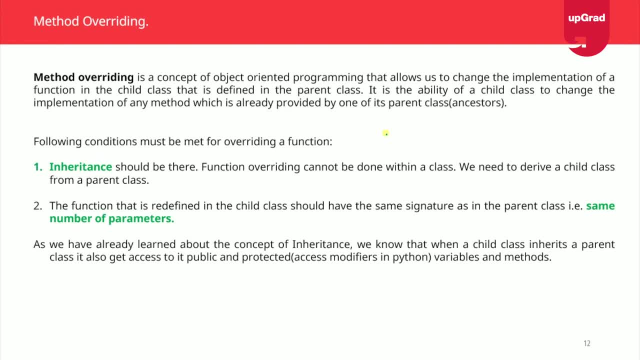 polymorphism. in simple words, we can define polymorphism as many forms, so here to define it in it. in other words, we can say that if any object has a capability to to represent itself in various forms, then we can say it: it has the capability of polymorphism. 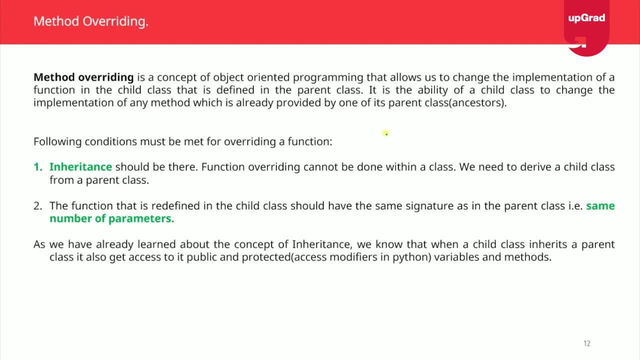 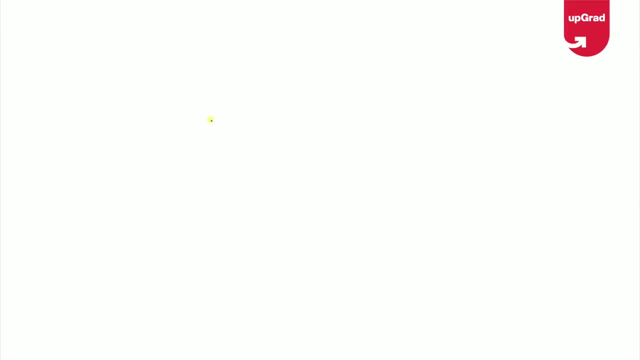 polymorphism helps us in representing the various states of an object in different forms here. so to understand polymer polymorphism clearly, let us try to understand what method overriding is now in method overriding. basically, what we do here is: we will call it- don't start with four days. we call it 자연, Chernoff one day. 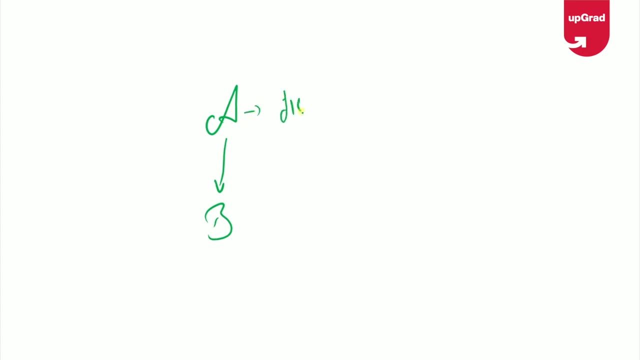 and also recognize at the time when your object changes in a different form. we also know that there are multiple ways to measure pero type cases where I am going to take aào, just set it as are this: f1 in the derived class, then this is called overriding. let me repeat: 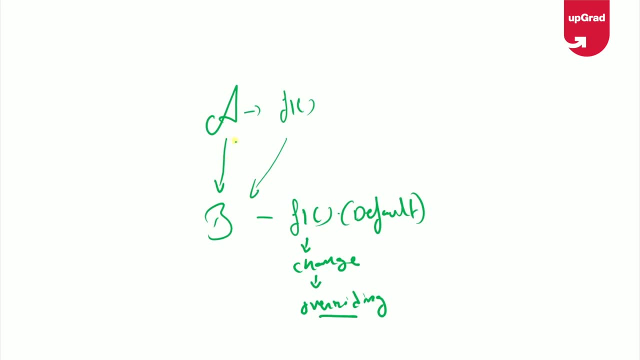 myself. so here suppose we have two classes, a and b. a has got a function called f1. now, due to the inheritance, this f1 will be available in B as well. by default you will get the default implementation of this function. but if you decide it to change later than this changing of behavior of the function in 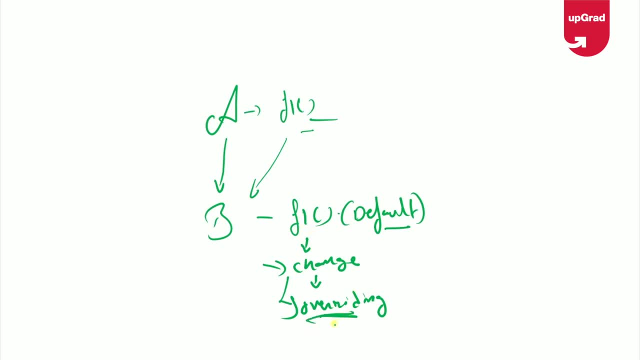 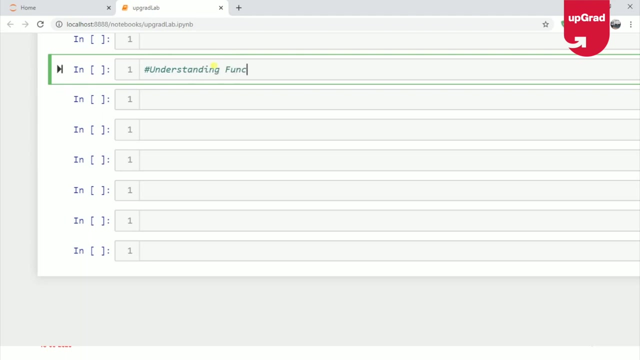 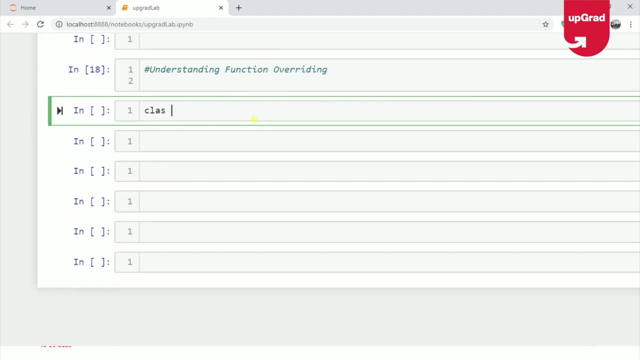 the derived class is called function overriding. let us try to understand function overriding via a practical demonstration here: understanding function overriding. so, in order to understand function overriding, let us take an example of a class here called father. now here we are defining a function in the derived class called function overriding. so in order to 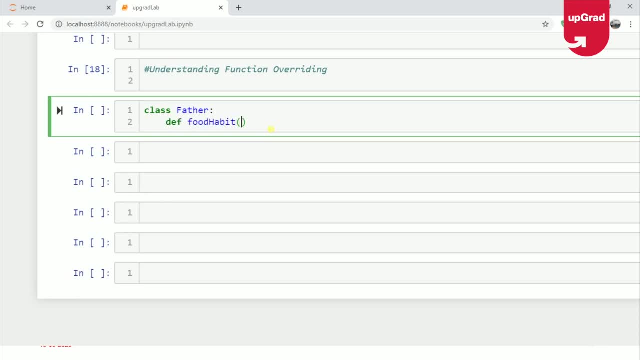 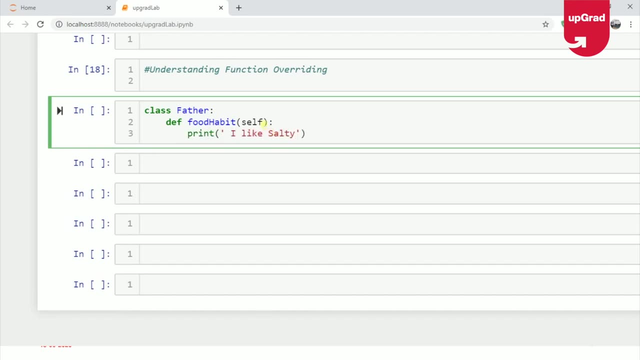 understand function overriding, we have to define a function in the derived class and that is food habit. so here you can see that food habit function prints a message called I like salty. so in simple words you can understand that the food habit of the father is that he likes salty. now we have a class called son here. 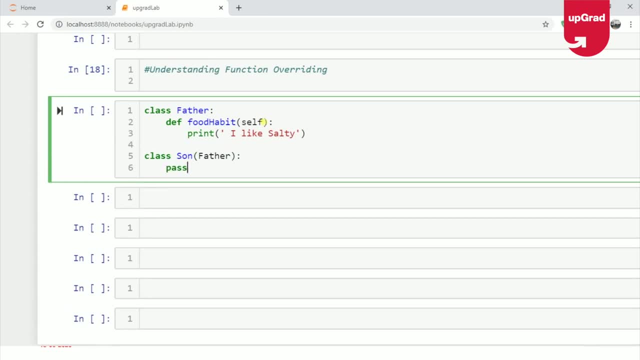 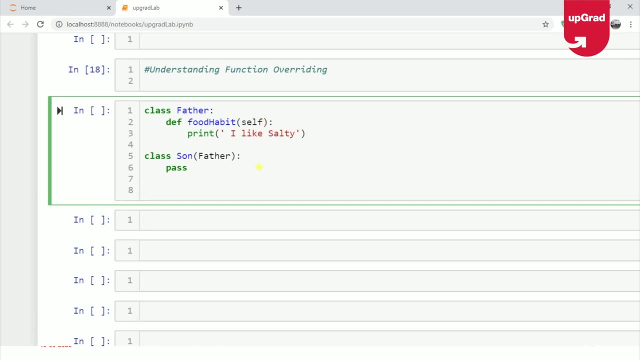 which inherits from father, and we are keeping it empty and, to prevent the compilation error, we're using the parse keyword here. now, because of the inheritance, or due to the inheritance, this son must get the same function: food habit in itself, the default functionality of this food habit within 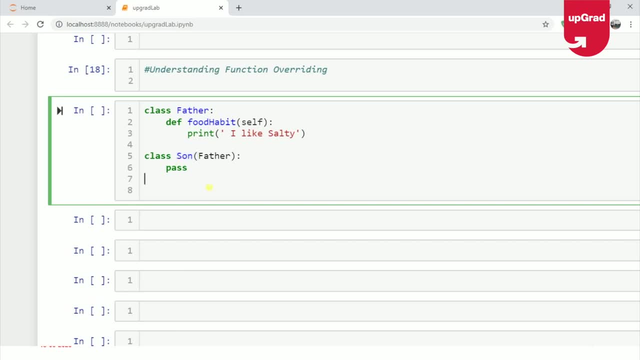 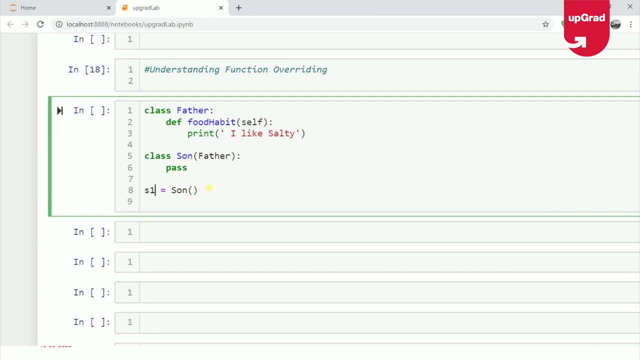 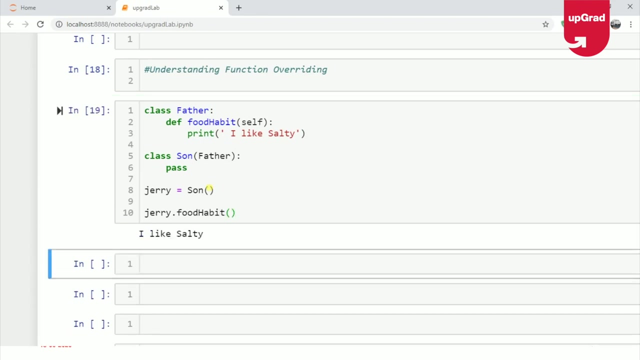 the Sun class would be. I like salty. let us try and check it, so I'll just call it Jerry. Jerry dot food habit. so if you look at the demonstration here, you can see that by default the food habit of Jerry is same as his father, which is the. 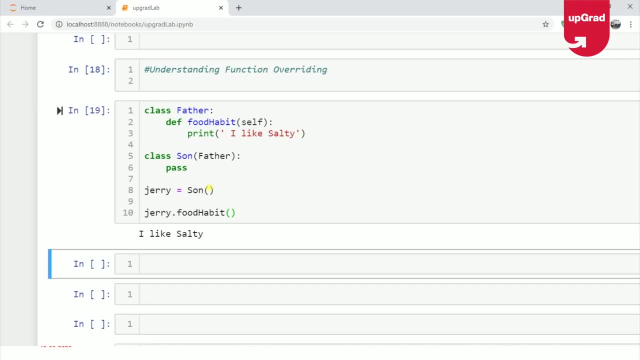 default behavior which is salty. but let's say the son decides to change this habit and now we will implement this food habit with a different taste here, which is sweet now, if we redefine the function which is sweet now. if we redefine the function which is sweet now if we 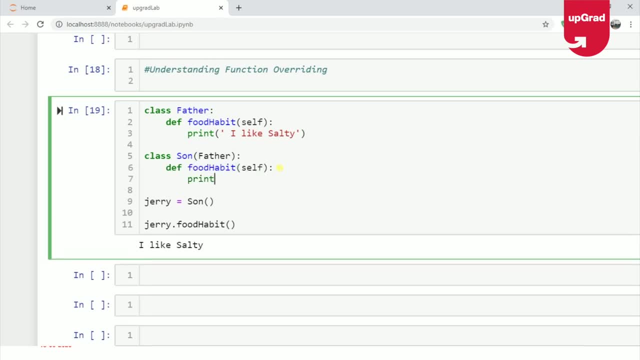 browse on to our database on the sizefuldot pop function or writing means. it means that the function of the function which was received from the parent or the base in the database is mod souce that we are diez تو do and ah derive class. so here you can see that I am red defining the function. so this redefinition of the function which is being provided here in the they're at us, this implementation is 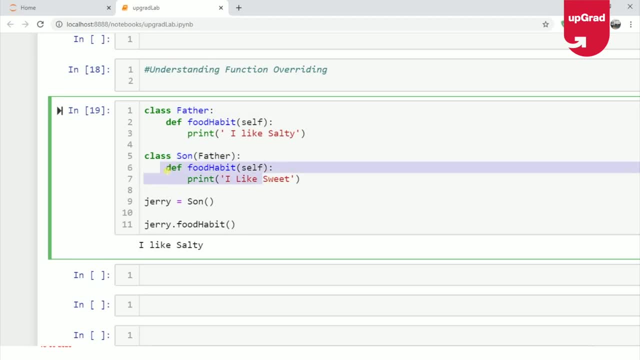 so this is function overriding. now here, if you look at the output, it says that I like sweet. now you need to remember two things here while implementing function overriding. one is that function overriding can only be implemented when inheritance is there. without inheritance function, all overriding is not in cannot. 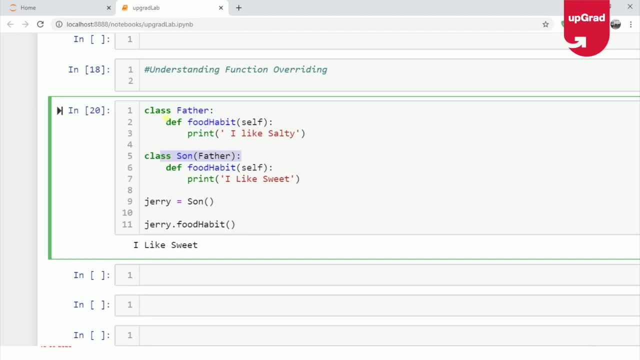 be implemented. second is the access of the function, and the base class must be same as derived class. all right, so function overriding is an example of polymorphism. so, as I explained you earlier, polymorphism basically means that many forms- so here the function, food habit- is existing in two different. 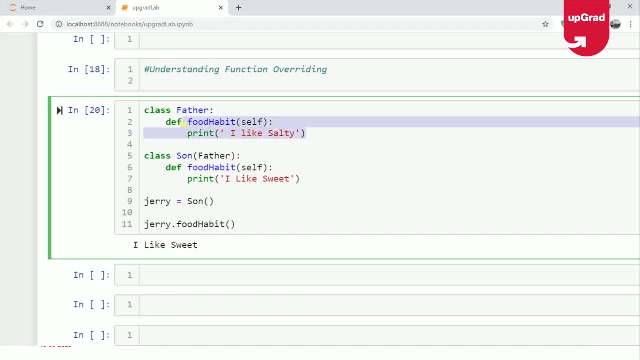 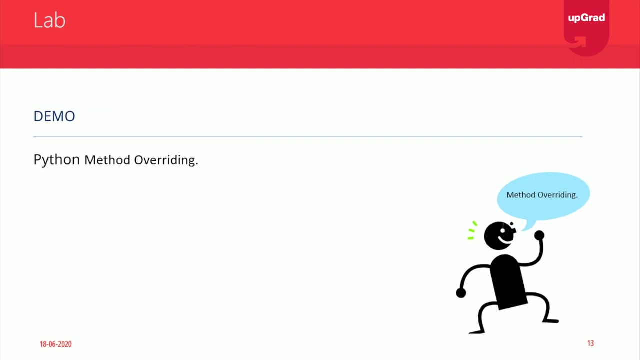 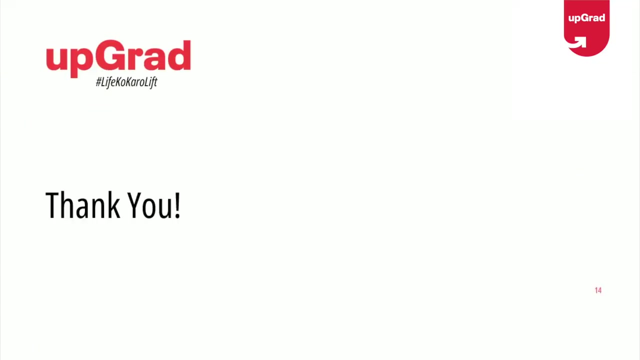 forms here. so here, the very first version of food habit is salty and the second version of food habit is sweet. so I hope that makes sense. you clear about understanding what polymorphism is and what is method overriding. all right, thank you everyone. so if you liked the explanation of our